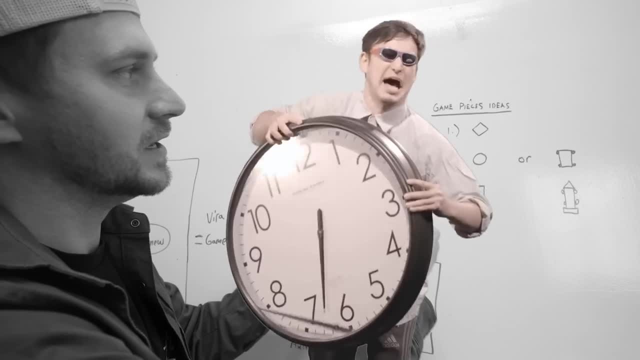 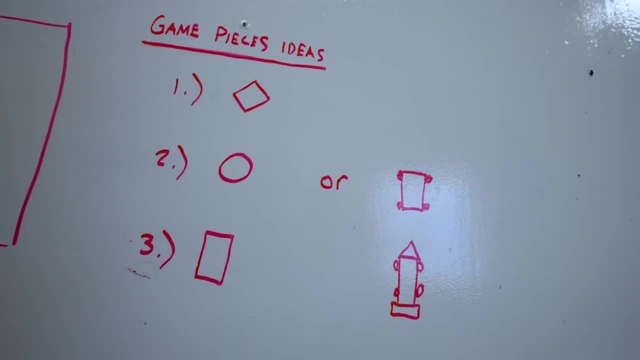 It's time to stop. It's time to stop. okay, Now for my game piece ideas. we have a triangle, circle or rectangle, Or something with wheels, like a car or a train. I'm thinking sports. I like cards, dice and boards. 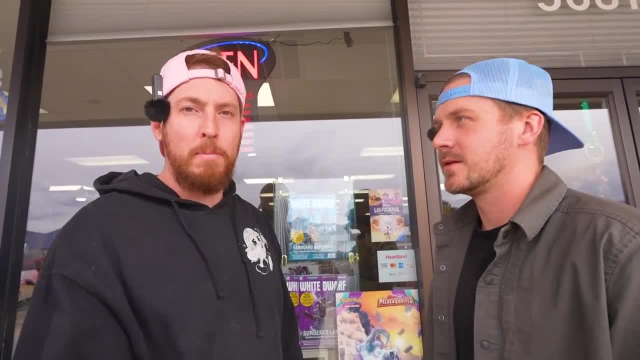 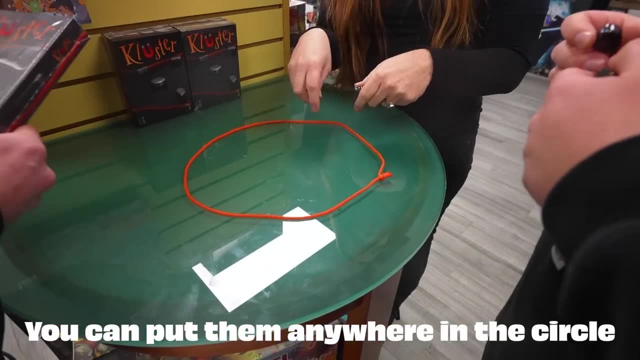 I've got it. If we want to make the best board games we can, we've got to go to where board games are sold. We need inspiration. It's pretty simple. The goal is to run out of magnets first. okay, You can put them anywhere in the circle, but we're going to put them down. 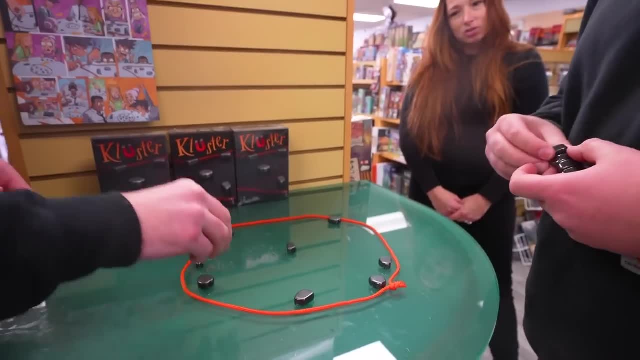 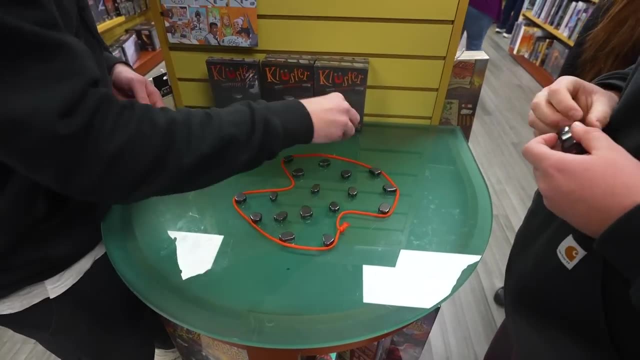 If they click together, that means You have to pick them back up. So what happens there? I have to pick that up. Pick that up. No, Ooh What? There's no way. those connected. Oh, that sucks. 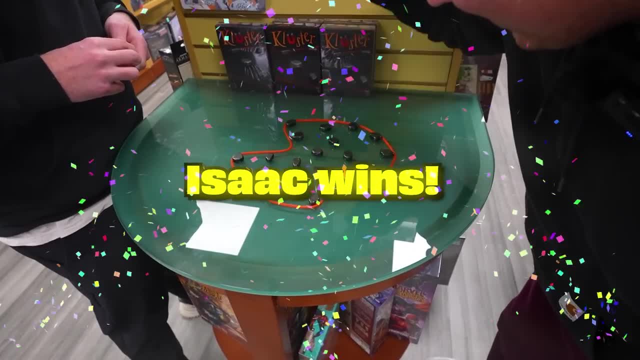 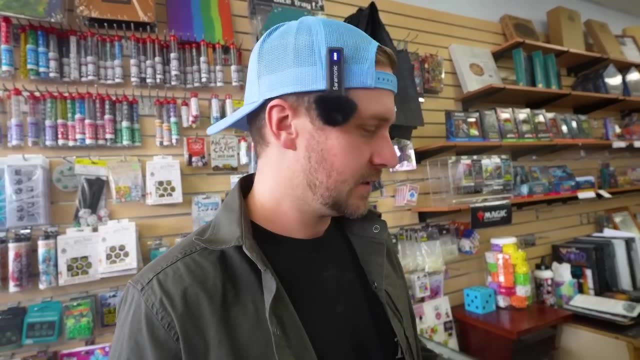 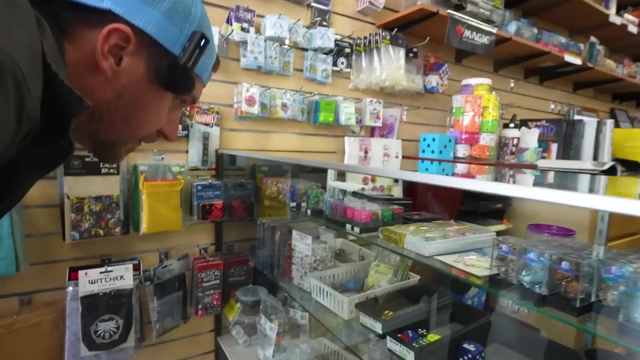 My last one. Ah, you bested me at magnet rocks Good game. My board game is going to involve dice and we have an amazing selection of dice here, So I'm going to get either two, Two or four dice. So I've got to find the best-looking dice which I like, these big fellas. 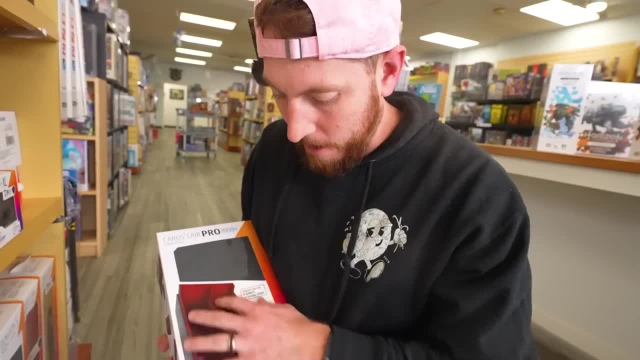 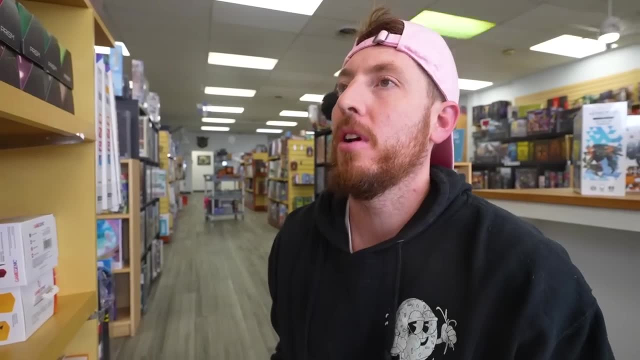 That's kind of fun. It would be sick to get this giant case to basically hold all of my game parts in, But this thing alone is $90.. Remember, our budget is only $200.. I think I want to utilize cards in some way, so I'm going to get this card holder and 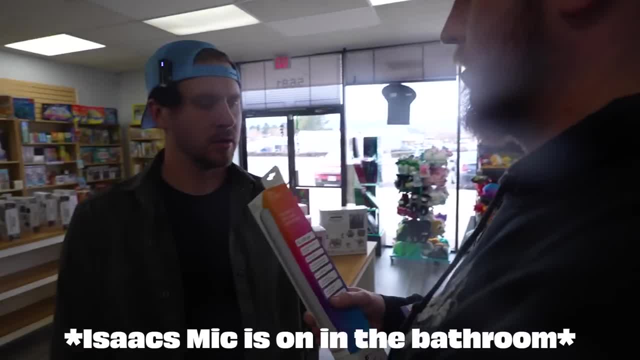 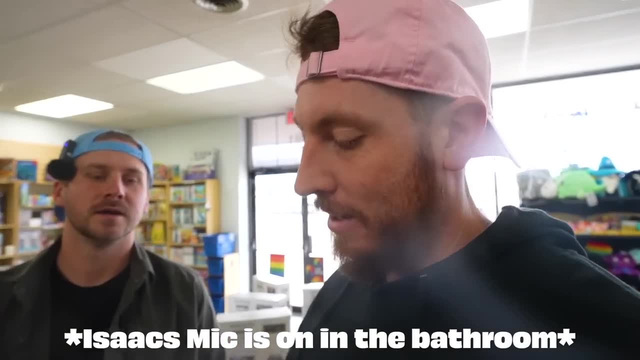 probably make my own cards. That's as far as I've gotten so far. What's your favorite board game? Oh gosh, El Dorado, Ooh El Dorado, I like El Dorado. Yeah, Do you want to make a board game based off stuff that I like, or one that's like this? 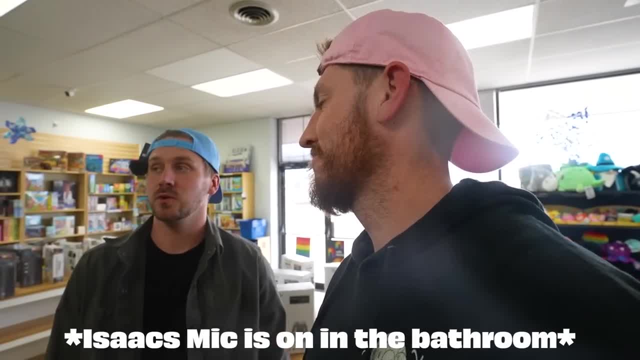 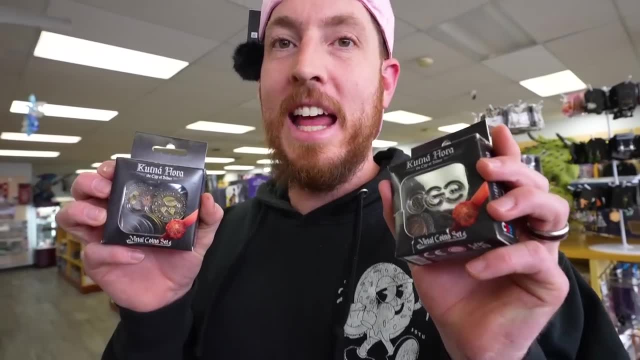 should just be fun, no matter what. You know what I mean. Do you like simple games or a little more complexion? I think I want to utilize coins in mine. So I found these box of coins and she said I can have them for free because they're promos. 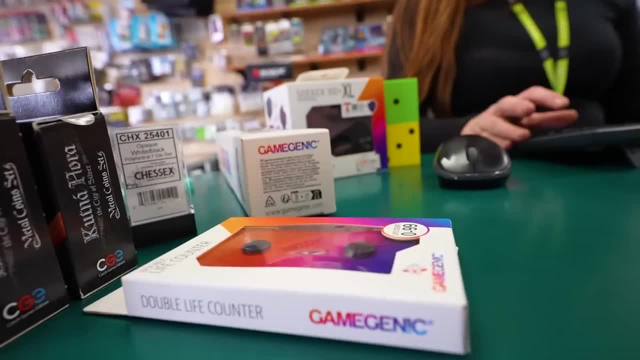 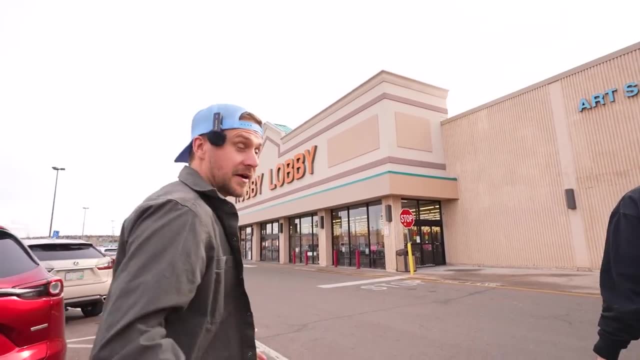 for the game. I don't know which game it is, but I just need the coins. It's now for my game: Hobby Lobby- craftsman's paradise. We are here at Hobby Lobby because we need to actually get crafts, because we're not. 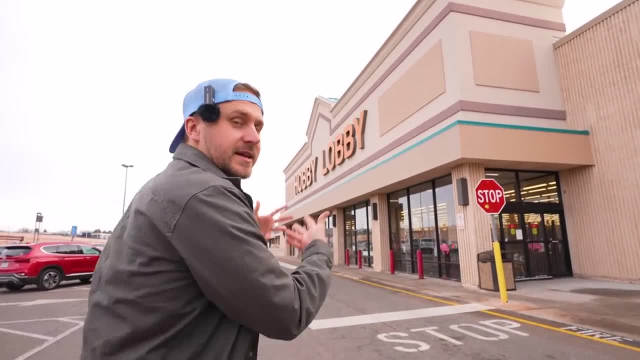 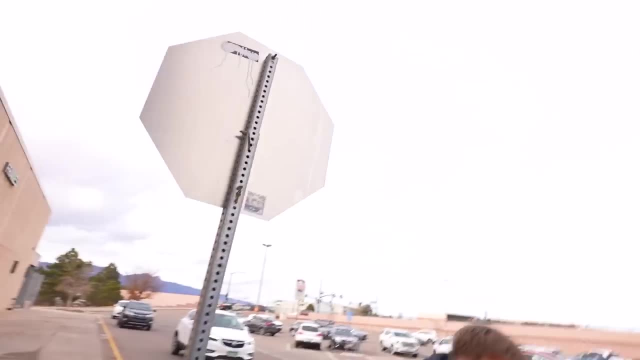 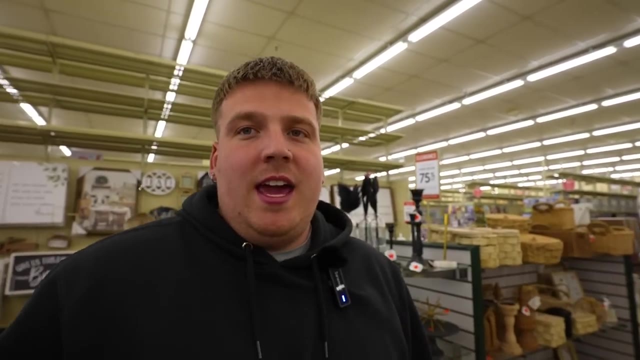 just buying a board game. We're actually making. it Need supplies. Yep, How much money have you spent? I've spent like $6.. My plan is to be somewhat of a sports version of D&D, So you're going to be playing a game. 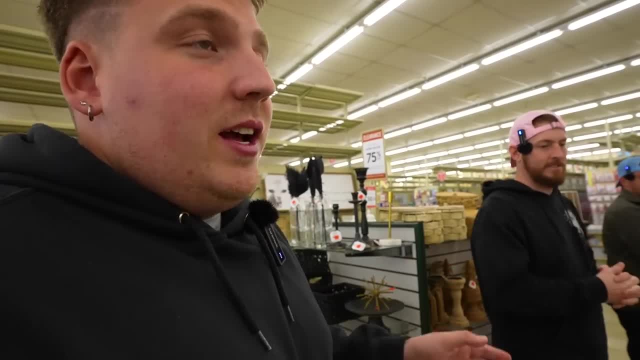 My case is going to be soccer, because that's the sport that I grew up playing. You're going to get your little players on the pitch and whatever you roll is going to dictate if you score, if you tackle all that kind of stuff. 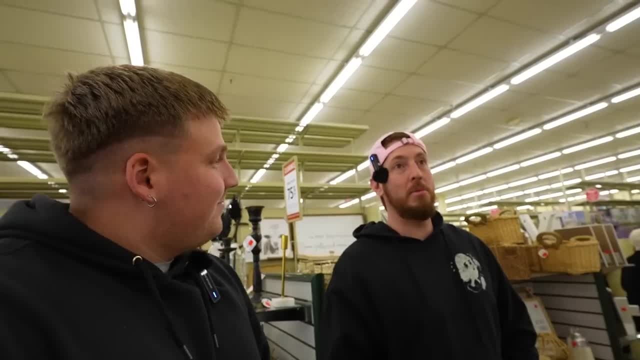 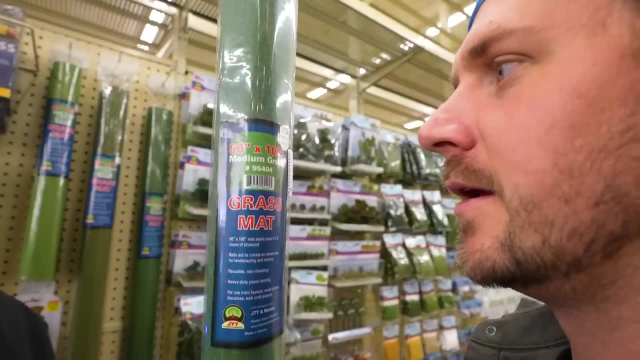 I'm still working out the rules Right now. I need supplies to build the field. I'm looking for almost like a case or a box or something that I put all the parts in. You found what I needed. I found what I needed that you're holding. 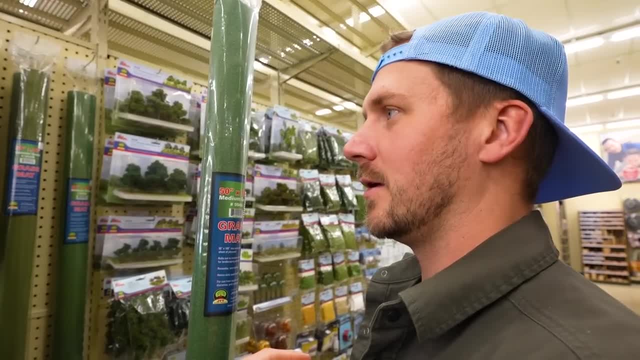 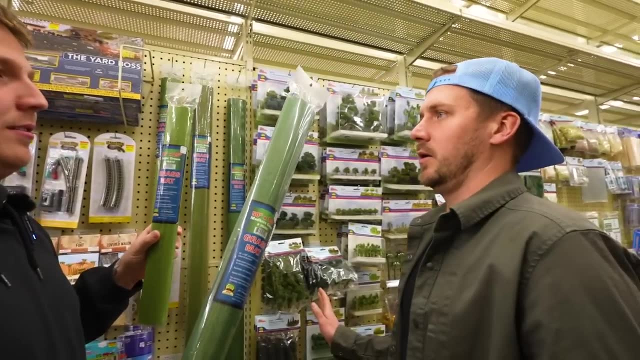 You found what I needed. You found what I needed, and then I found it in your hand, Me holding what you needed. I found you holding what I needed. This one actually might be the perfect size. I don't want what you want. 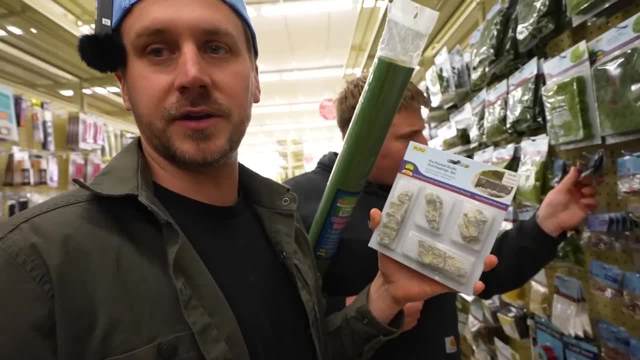 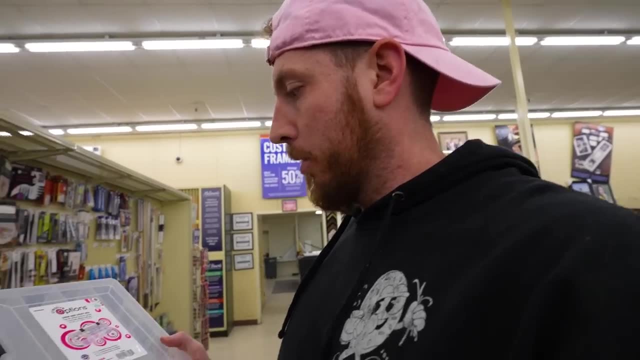 I'm making actually a cool map for my game. I know you guys still don't understand what game I'm making. Having these fake mini rocks is going to be very good. I found basically what I'm looking for. Look at this storage bag. 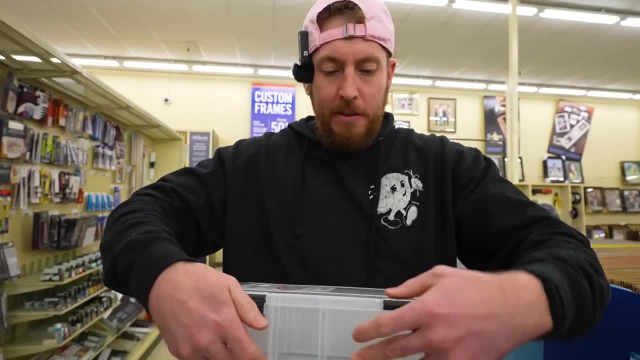 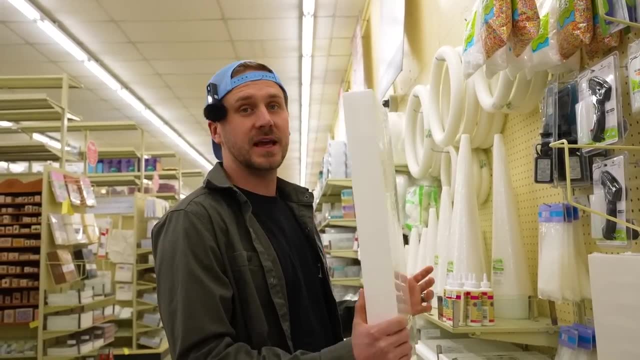 Put the playing mat here, the cards, the coins, everything in one bin. This is a phenomenal game board base, so I think I'm going to get some of these. This will help me put together my map Walking around Hobby Lobby. I feel super human, creative right now. 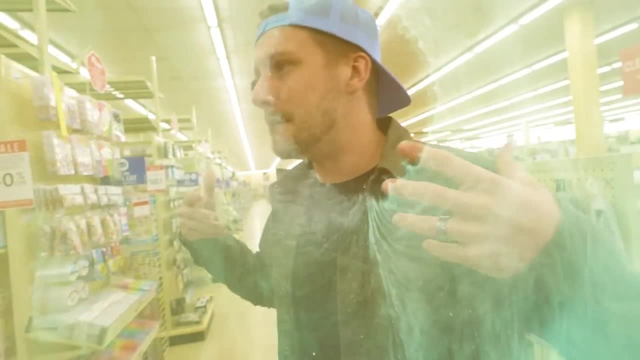 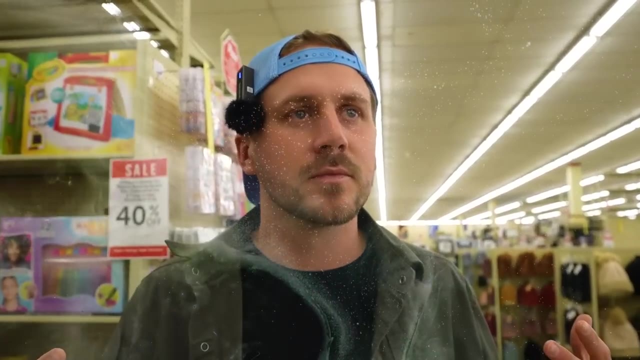 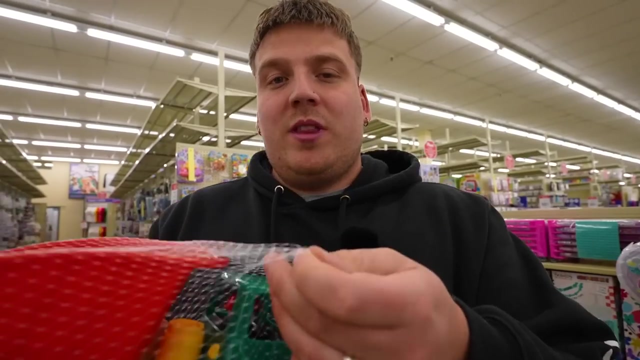 Every aisle is full of ideas and spawning new and better ways to play my board game. I'm about to explode with creativity. There's probably some sort of effect that happened there. Guys, I don't actually want this truck, but I do want the packaging. 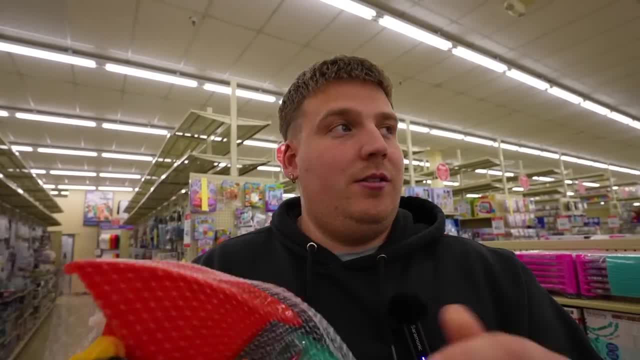 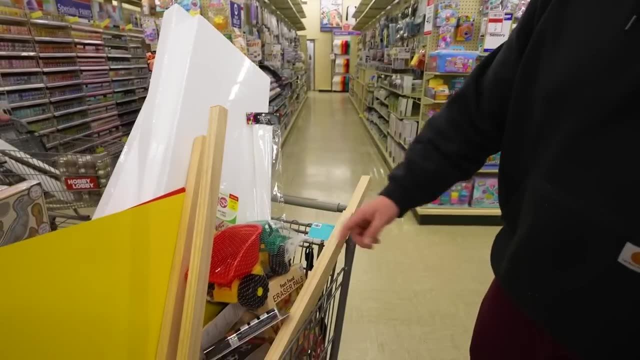 This is going to make the perfect net for the goal, and so it's only seven bucks for this whole thing. Worth it, I guess. Yes, Good, Yeah, Rick is going to love this truck. All right, we're at the Iron Lion. 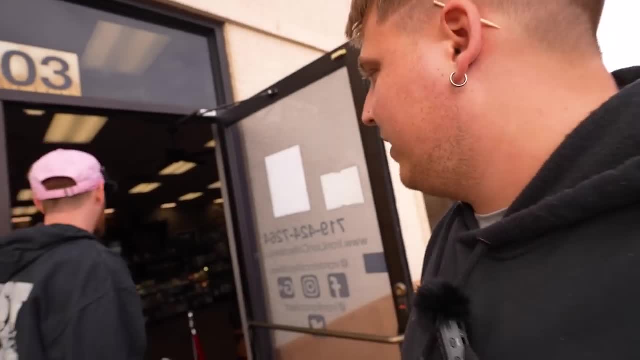 This is a trading card store, Comic book store And comic books, but they got trading cards and that's what I need, Guys, this is what I was looking for- the soccer tops cards- and they're only $3 per pack. so 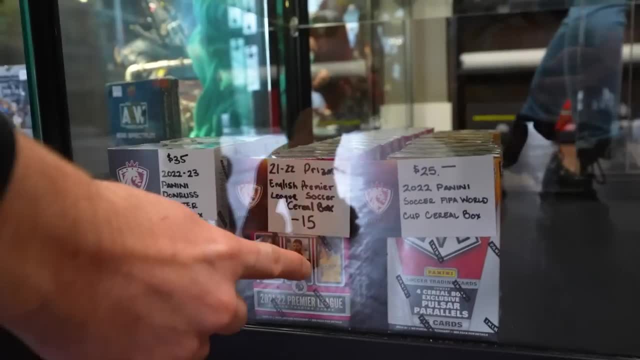 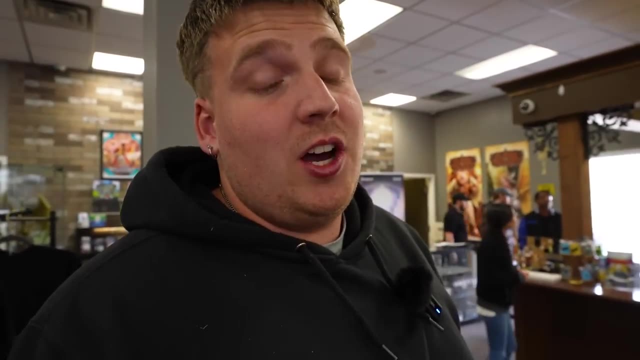 that should be fine, Perfect. I know the most about the Premier League just because that's what I watched with my dad and my brother, so it'd be nice to at least have teams and players that I know the most about. Guys, I'm buying four packs, which is $100, so I'm spending half my budget on these cards. 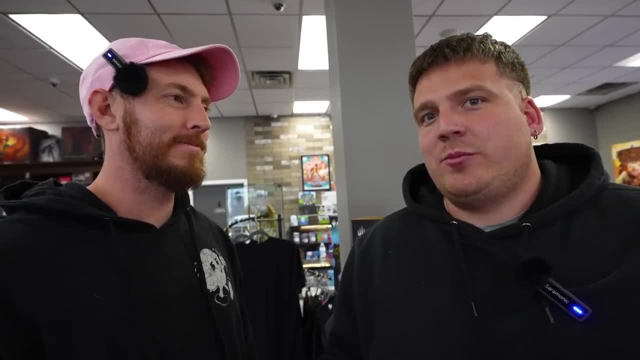 because that's kind of what's going to give this game the dynamic. Every match will be different because you're getting different players, so it'll be pretty cool. I'm not going to say this to the judge, but I really want to play your game. 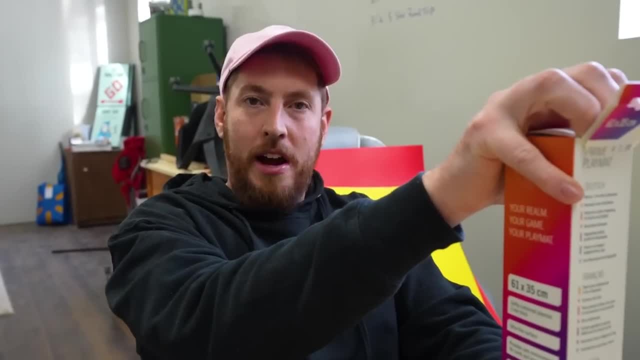 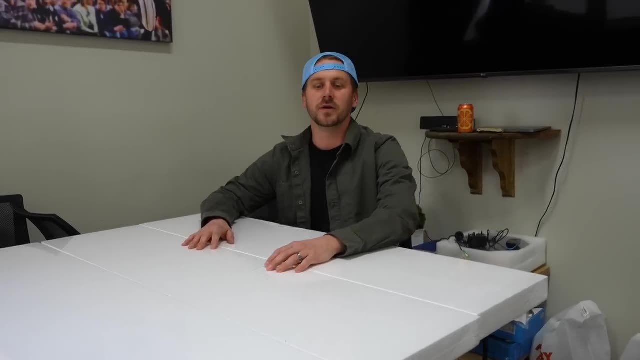 Really, Yes, Heck, yeah, We're back at the office Time to start designing these board games. Oh no, This is my game board. Oh, I thought this was way bigger. Here's my game board. Actually, just one of my game boards. 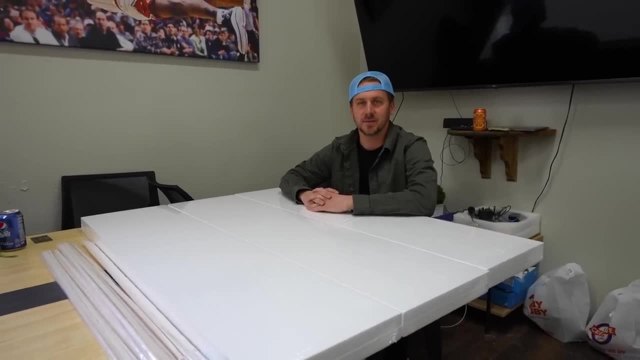 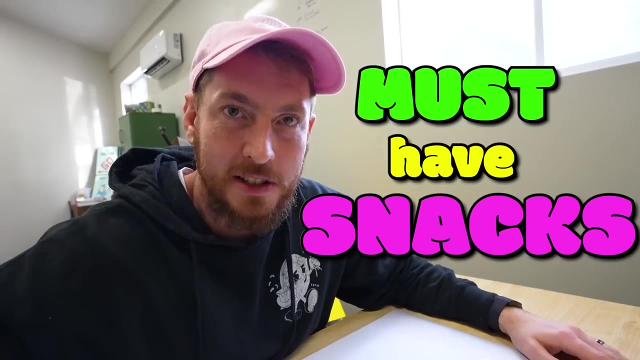 I'm going to have two different variations to my game. I've got these blank cards, so I'm going to make a whole bunch of unique cards. I'll already tell you the title of my game. It's: Must Have Snacks. The Game. 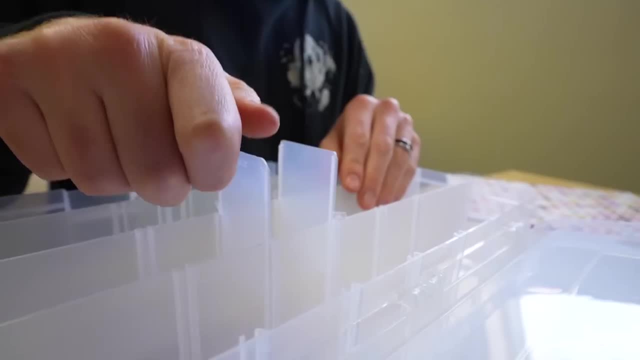 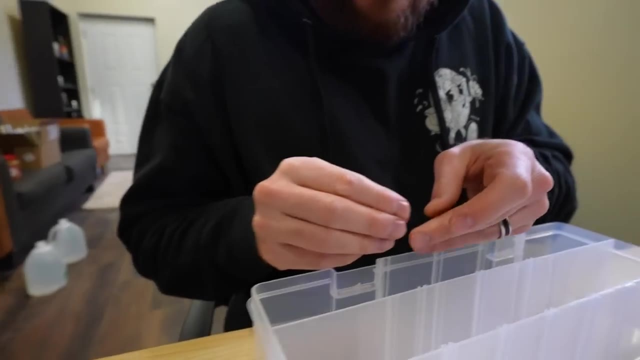 All rights reserved in the attempt to copy or distribute this product. These need to go all the way in. Ah, it's stuck now. It can't be normal. These will be coins for my game. These will be the starting coins. Every villager gets one. 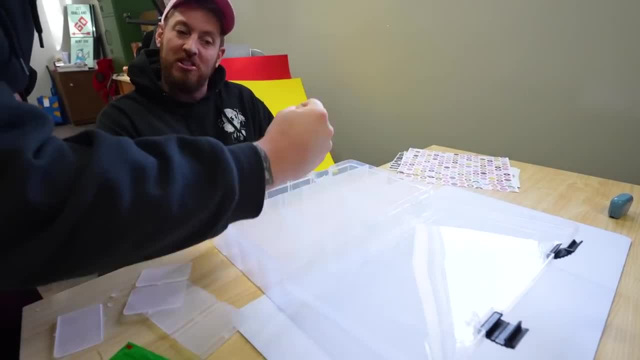 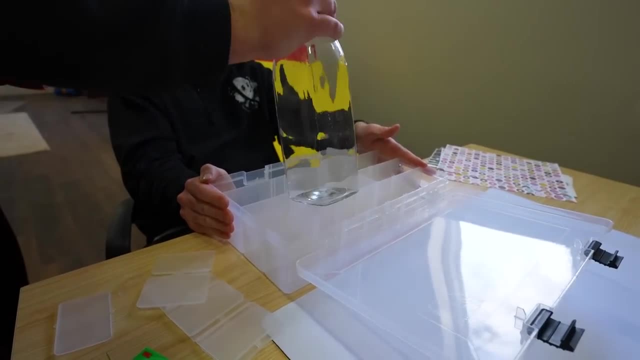 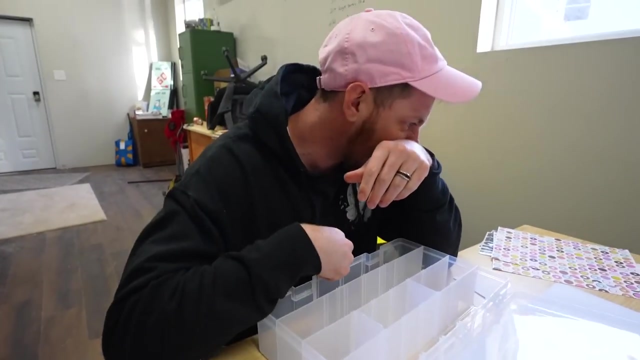 Ow, How'd you do that? What are you going to do instead? Oh no, Clearly something's wrong. Now my case won't close. My game's ruined. I give up. I know you guys are wondering just what exactly my game's going to be about, and I just love. 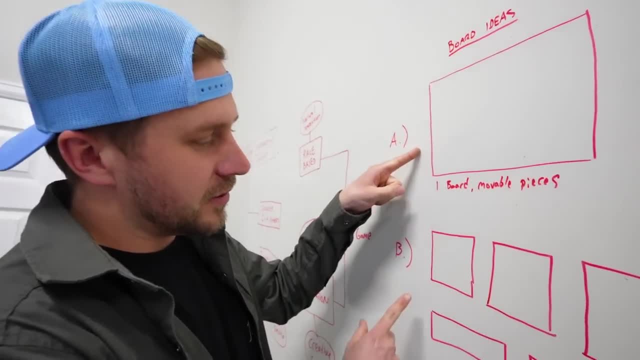 keeping you guys in the dark, because this is going to be incredible. Remember this plan, Remember what I said earlier: I'm actually doing both ideas, So I'll have one board and I'll get to try them out. I'm going to install my first board. 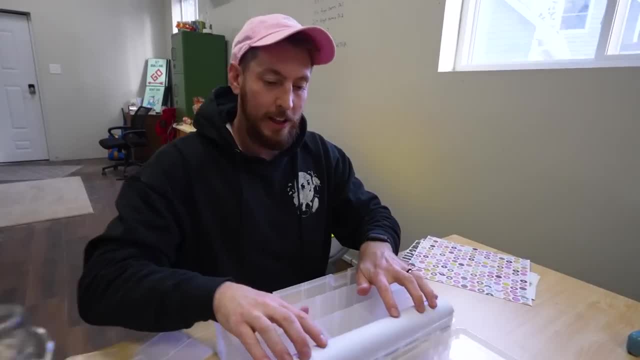 It literally fits perfect. If it was any bigger, this box wouldn't work. It's the perfect fit. Ow, I am attaching my fake grass to this long board. It's going to be actually a pretty big game. It might be the biggest one. 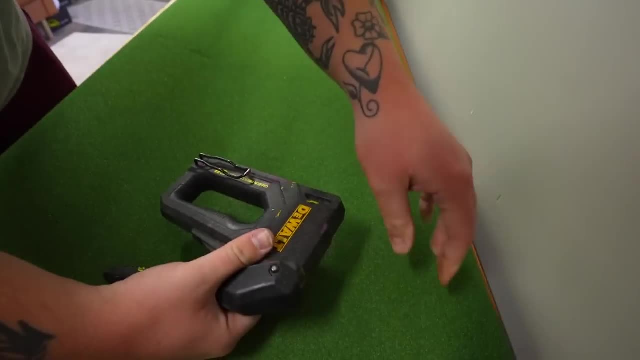 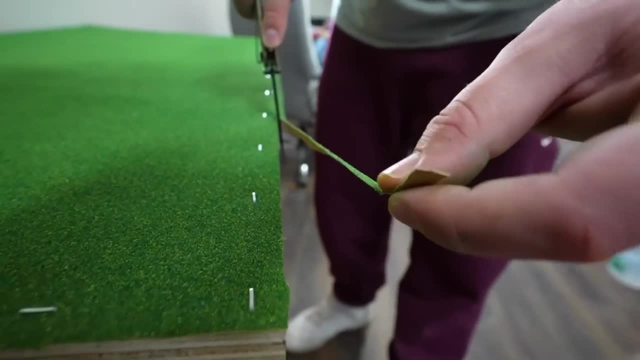 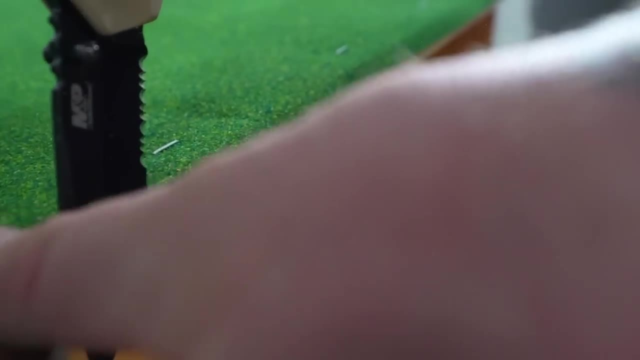 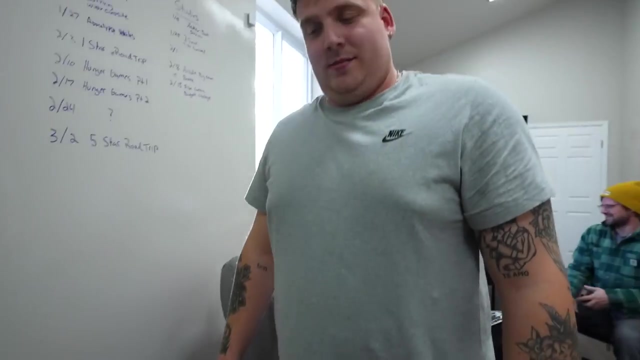 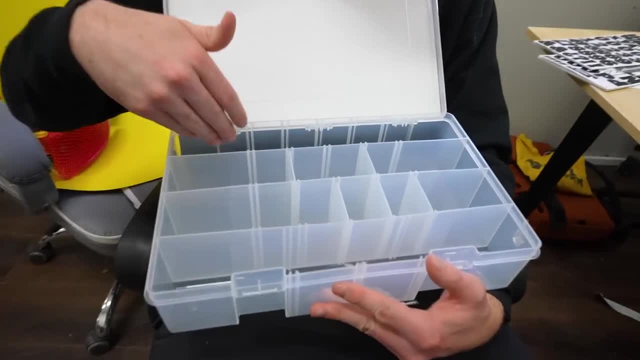 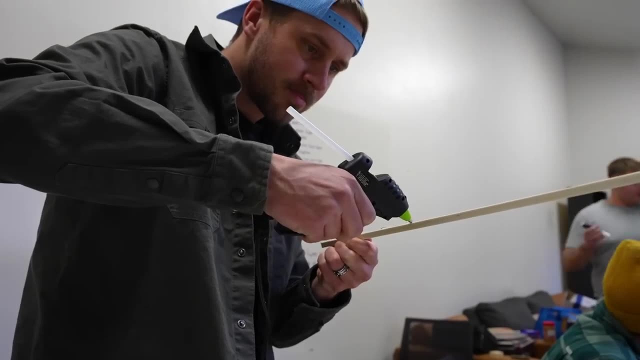 ever Comment. now I think I finished my game box. I got the playing mat, The cards go in here, The coins, All stuff's. next The game. I am hot gluing my game board together right now. Hot glue is clutch whenever you need just something to stick fast. 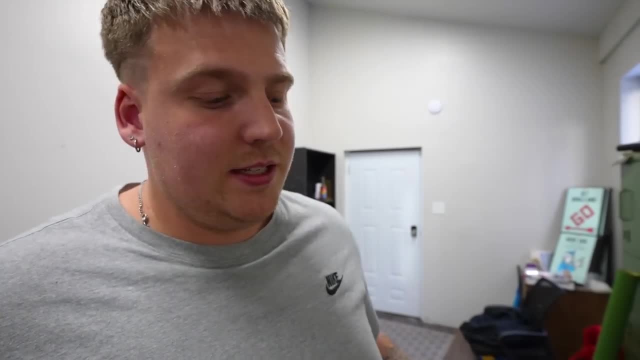 Highly recommend This paint pen and I thought it would be the perfect thing to do the lines on the pitch, but it's not. I'm going to just restart. I really want this to look good. I want to put as much effort as I can into this. 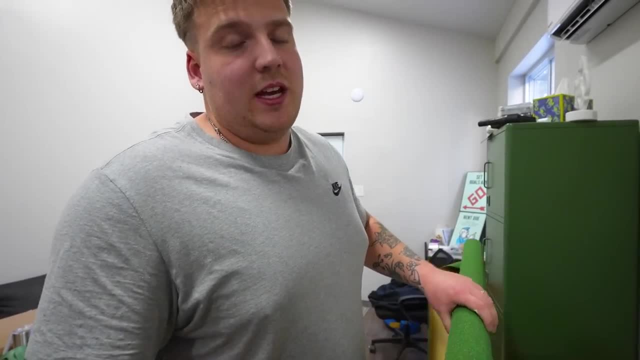 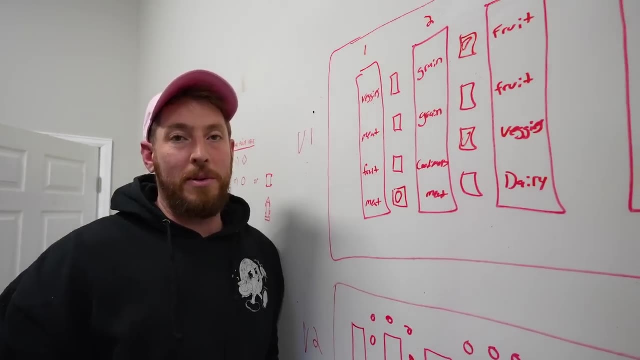 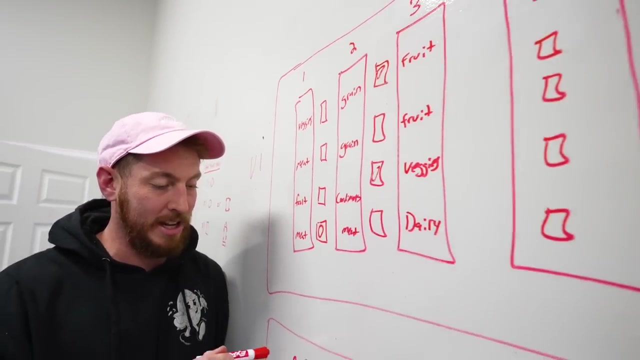 I have enough grass that I can kind of restart, and then I'm just going to have to use actual paint and a paint brush. So a slight setback, but of no, worries, I've been brainstorming some different variations of the Must Have Snacks game. 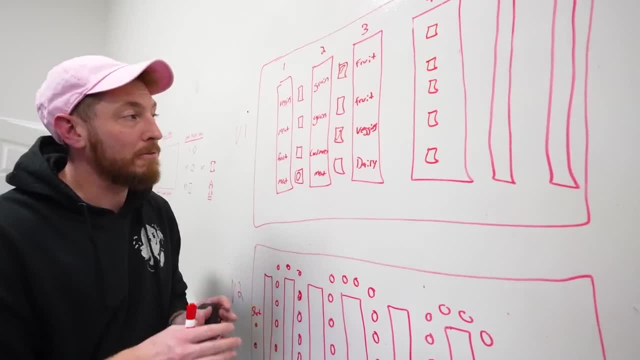 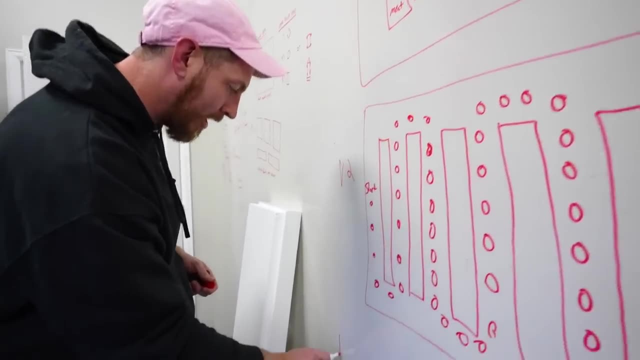 We've got version one and version two. They're coming together, but unfortunately neither one is fully fleshed out yet. I'm not sure which direction to go, or to keep working on, or if there needs to be a V3.. Right now I am placing my racetrack boundary line. 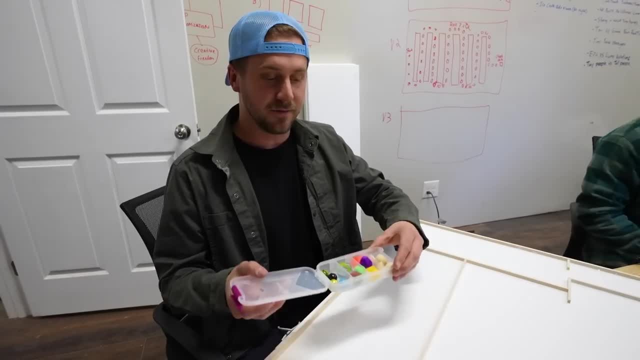 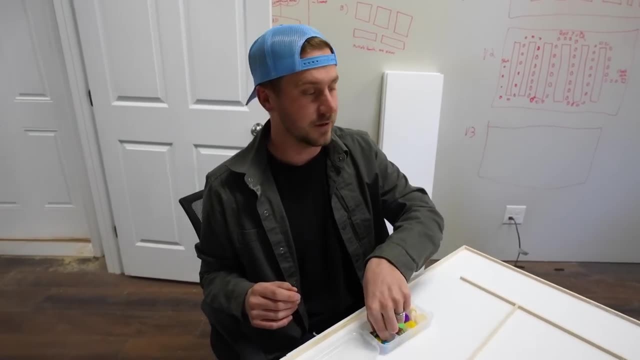 It kind of looks like a maze right now, which it kind of is- and I have four different game pieces for the race and I have a bunch of props I'm going to install as well, but this is actually pretty fun, All right. 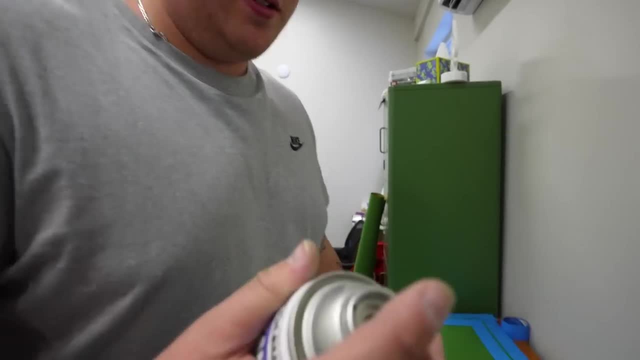 Take two. This time I've got spades, painters, paints, paint. This time I've just got spaders. What the I've got painter? This time I have painter's tape and spray paint. Hopefully this works a little better. 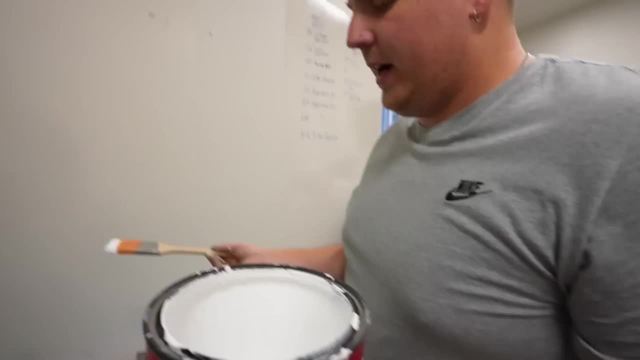 Maybe I should just use normal paint, because this is not going on there very well. All right, I finally got it to work. This is definitely the more difficult way, but there you go. Don't take the easiest way out every time. 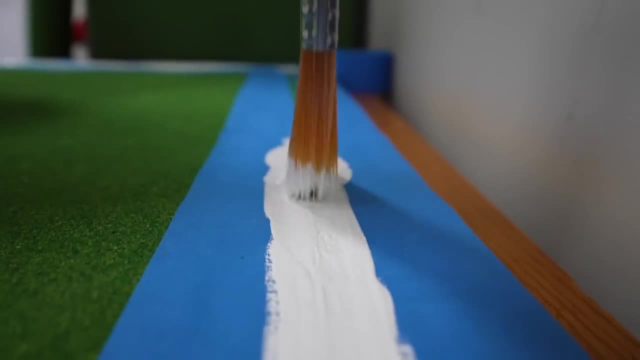 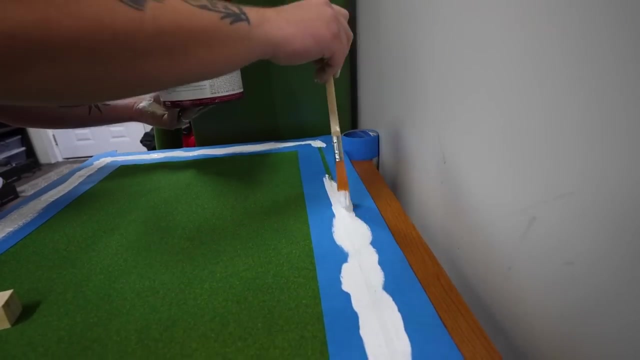 Spray paint would have been easier. Real paint better. It's going on nice and thick, giving me an actual, nice white line. I got to make sure I'm really careful I don't spill any on the pitch, Otherwise I'm going to have to restart again. 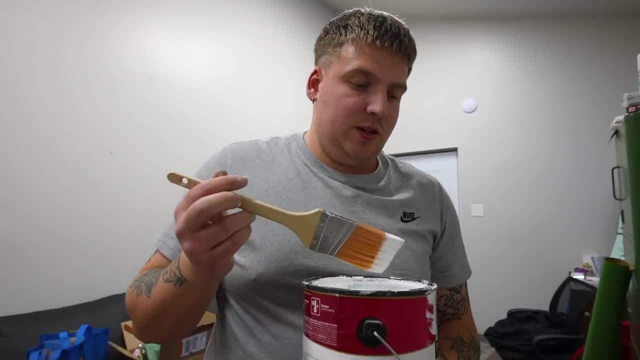 I'm going to have to let this dry and it's going to be my tester lines, because obviously I still need to do a couple more. I need this base outside layer and then I can use that as a reference for the rest of. 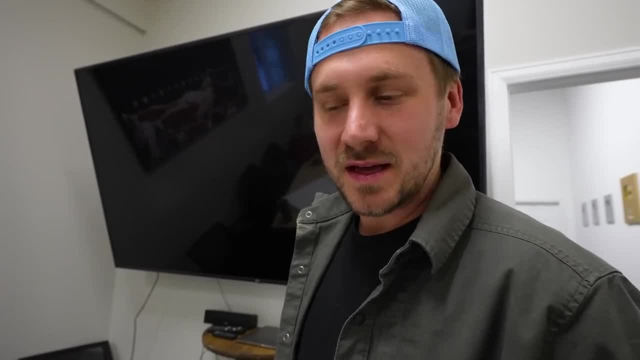 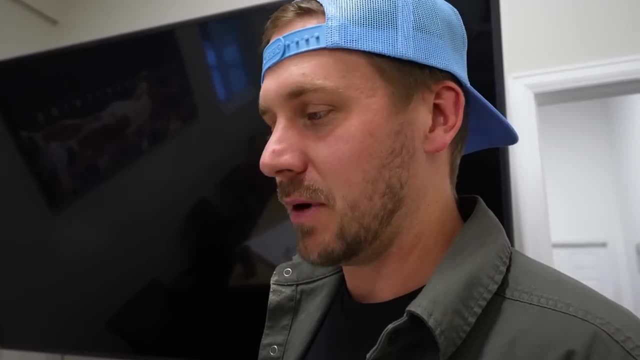 my lines. After I've been creating my map for a while now, I don't know if I'm going to be able to make a second map. I'm focusing on making my only map, the best map possible. I'm going to see if the paint line's dried and how it looks. 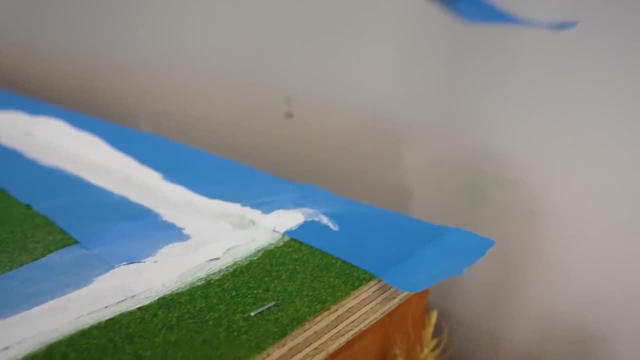 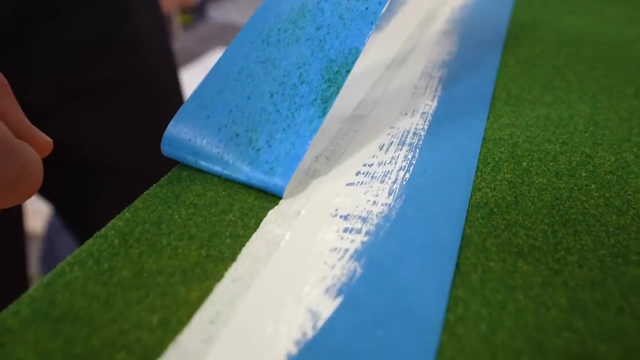 It's definitely dried. A little leakage, I guess, where the tape wasn't put down. Chloe, Okay, Let's see They're not pretty good. I honestly was hoping it'd be just a little cleaner, but I ended up designing the board. 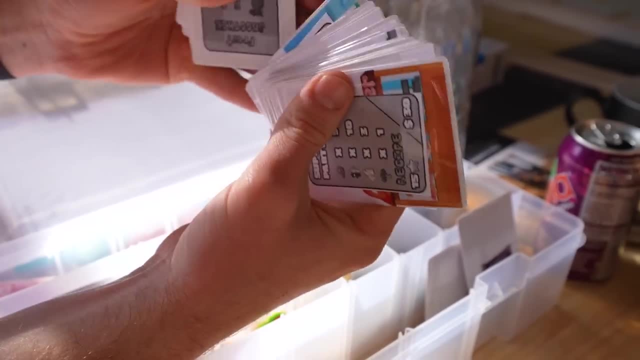 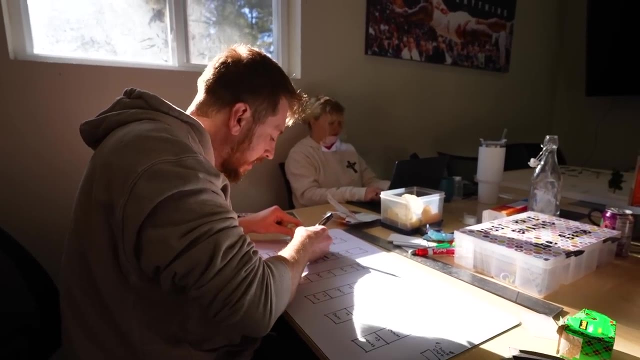 I made some more cards last night. Check these out: Whoa What Those are sick. actually No way, guys. Scotch tape. Remember: these are just prototypes, so if the board isn't even or there's something off, don't get mad. 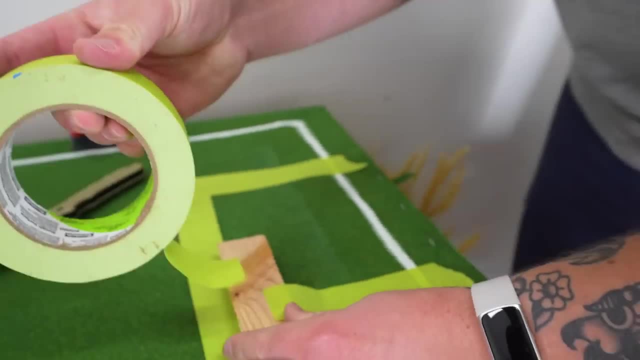 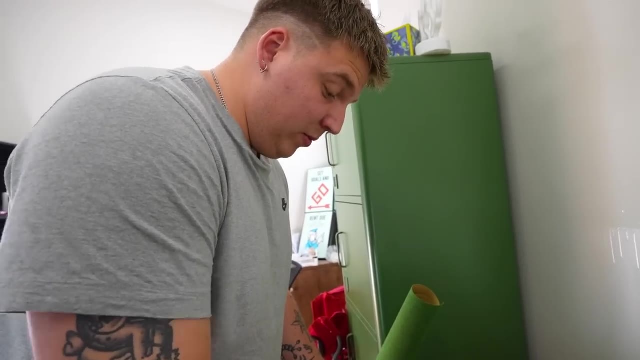 This is where things are getting a little more tricky: Making the cape as box Guys. I don't think I've ever put this much. I've never put attention to detail into a build before In my head. this game is so fun. 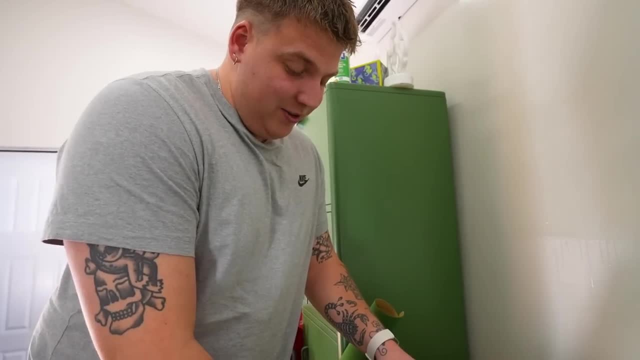 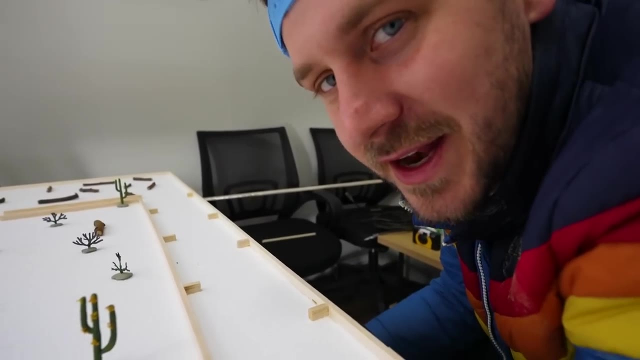 It's going to be super sick. I just want it to look perfect. I'm even using a tape measure. Can you believe that, Putting the final touches on my racetrack, This is coming along better than anticipated? I really need to get all the paint on so it can be dry by the end of the day. 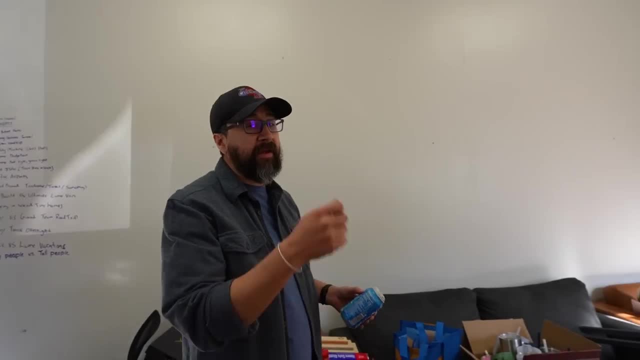 When you're painting cars, you do take it off. while it's a little bit tacky, Yeah, it keeps it from flaking off. That's what Rick says, That's what I do. Ooh, look at that middle line, baby. 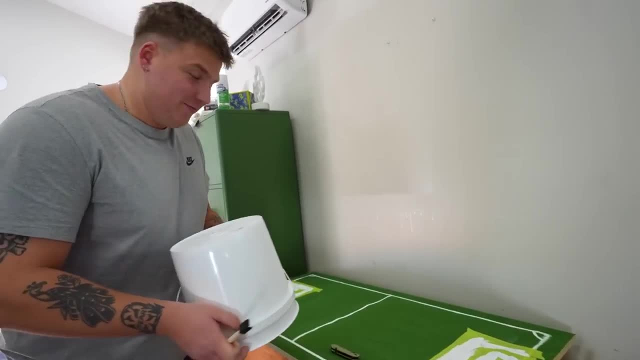 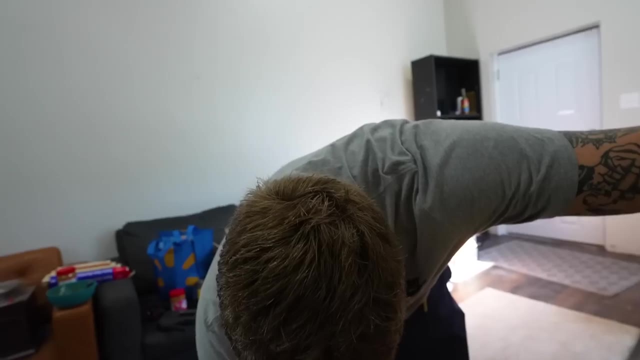 Woo-hoo, If I mess this up, I have to restart the whole thing. Maybe you should wait until it's dry. now, That's what I'm saying. I really need to get all the paint done Now. this is going to be very, very scary. 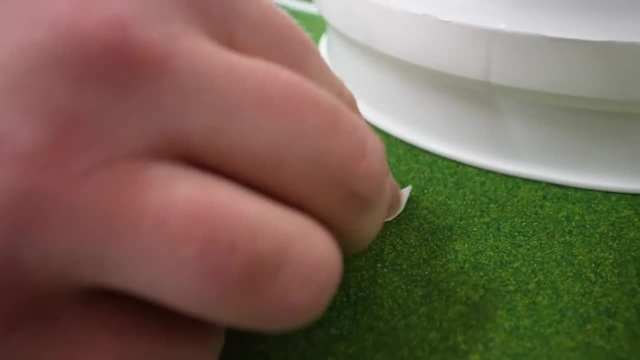 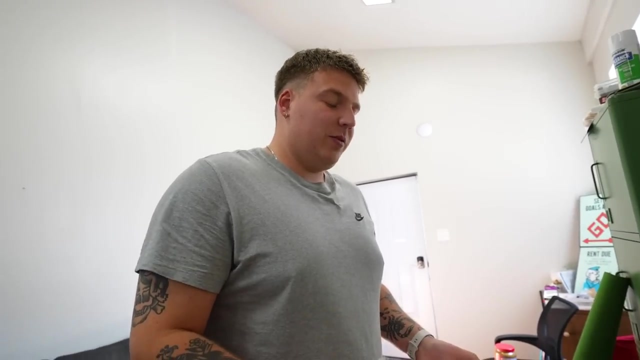 Oh, I can't believe I've done this. I can't believe you've done this. That is so maddening. It's actually not bad. Yeah, it's not terrible. I can't be too much of a perfectionist with this build, even though I want it to be perfect. 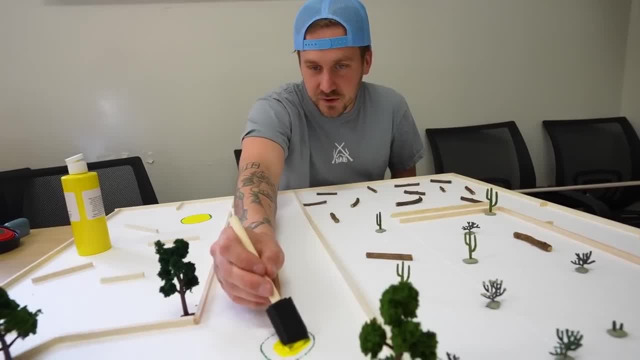 There are special zones where, if you and your racer are in the zone, you get to do something to your opponent. I think I'm done designing. I'm done designing the game board, so now I'm going to set it all up. run through it. 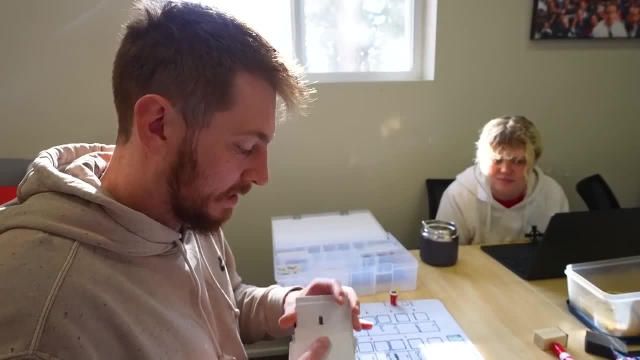 see if the rules make sense, if there's anything that needs to change- which you probably need to, I don't know, though, yet It's important to beta test your games before the judge comes. We're trying to complete these recipes. 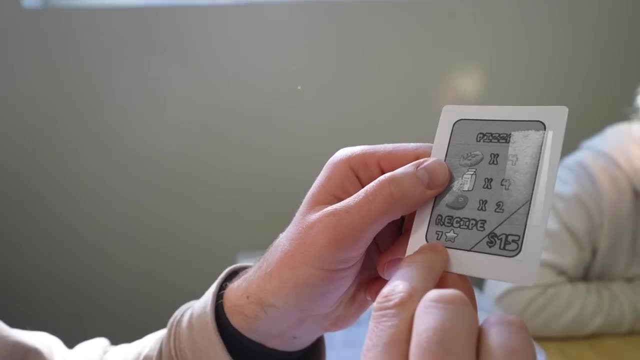 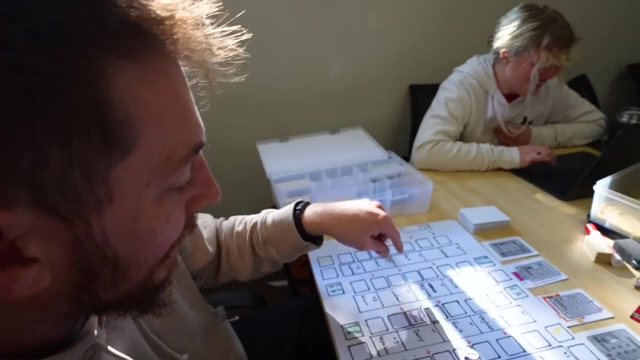 This is how much they cost to buy. so this one's 15 bucks for a pizza Gives you seven victory points. How many victory points do you need to win? Don't know. yet You're going around the grocery store and you're collecting the different ingredients. 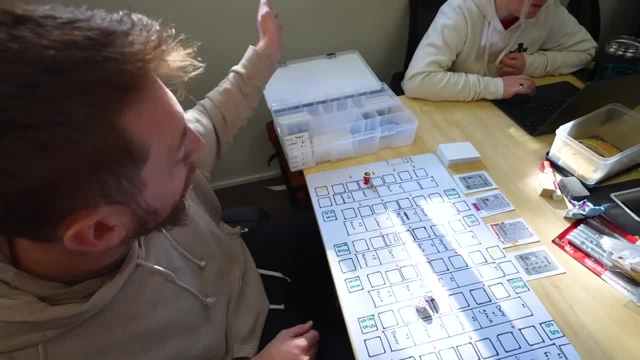 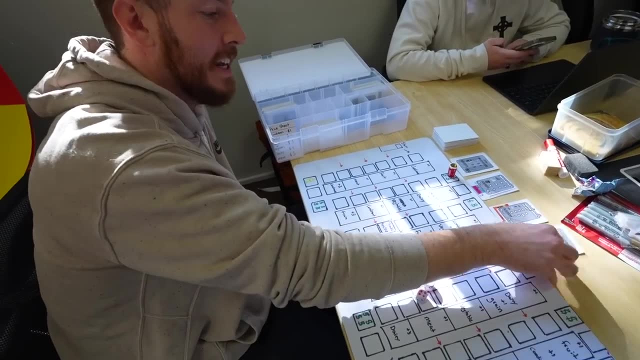 If you roll a seven, all your ingredients have expired. You have to put them all back and you're going back to the start. But if you land on one of these green squares where you can sell your ingredients, that's how you get money to buy your recipes. 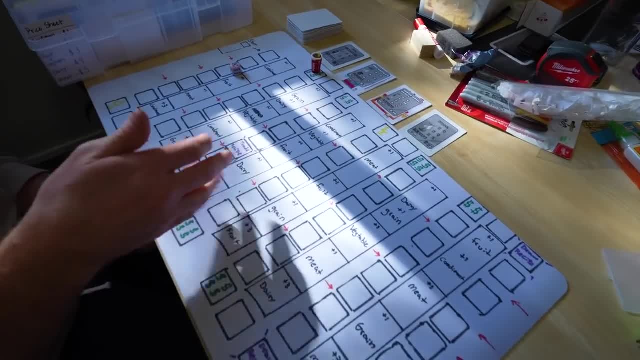 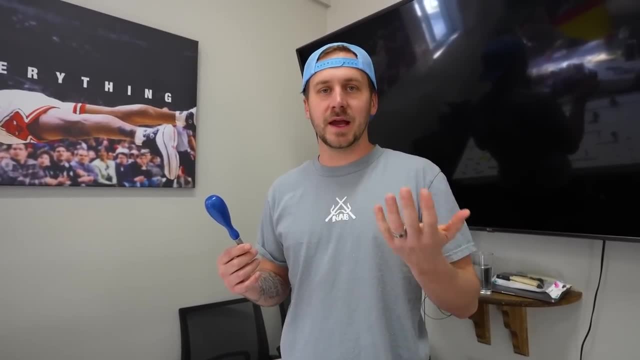 So it's very important to sell your ingredients, but then you also need ingredients to complete your recipes. So remember how I said my game could either involve the hands or sensory component. Well, I have both for my game. You can use your hand or you can use this device I got. 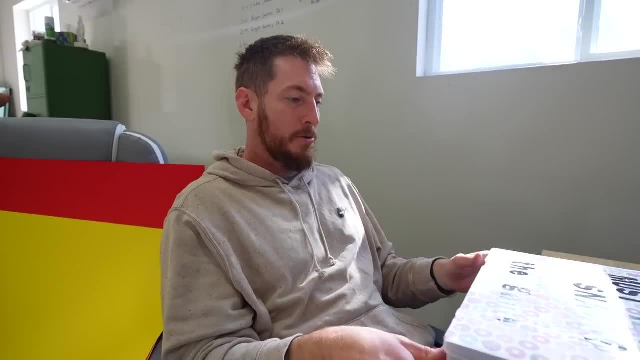 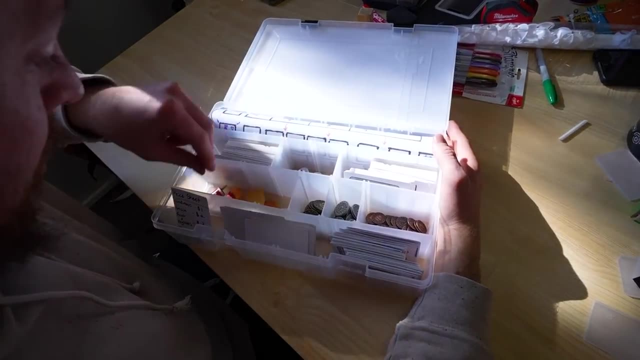 I've tested it. I think it works. I haven't run into many issues yet and everything fits into my box here. Everything has their own compartments. We've got the money, the cards, the books, Dice, The characters, Extra cards if need be. 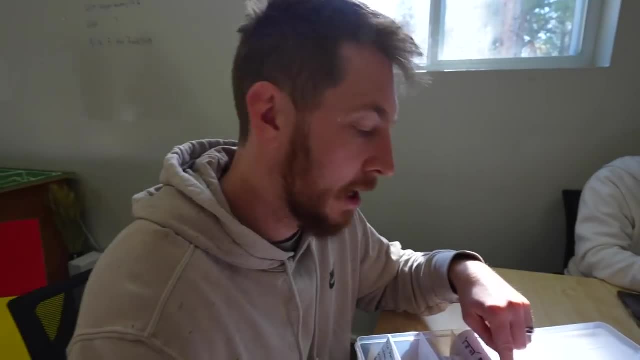 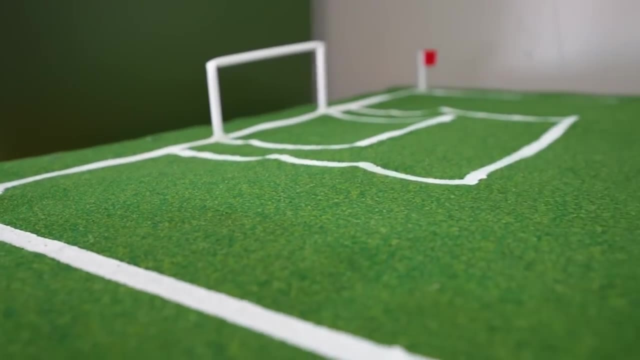 The price sheet. The game board Also. I don't know why more companies don't make squishy game boards. This fits so easily in here and when you roll the dice on it, oh, it sounds so nice. I'm going to open up these cards: see who we got. 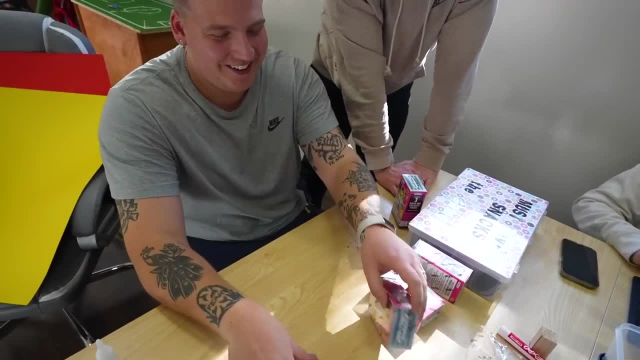 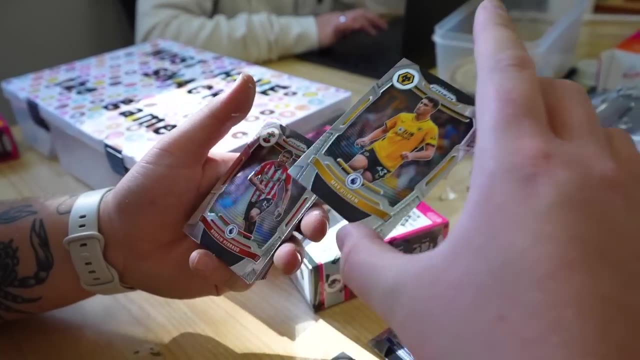 And Andrew really wanted to help because he loves opening cards. Josh Brown- hell, I'm a Liverpool fan, so I was hoping to get at least a couple of those guys. Townsend, These are some decent cards. Ooh, you got some specials in there. Isaac in the back. 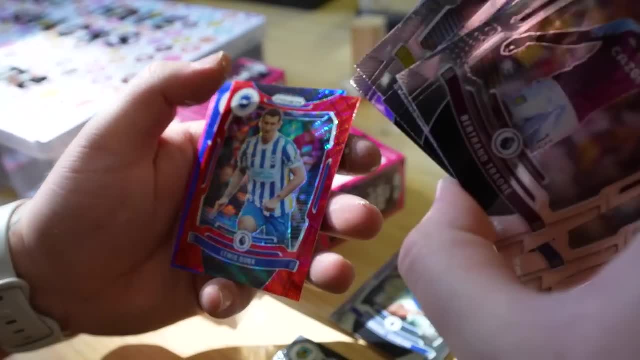 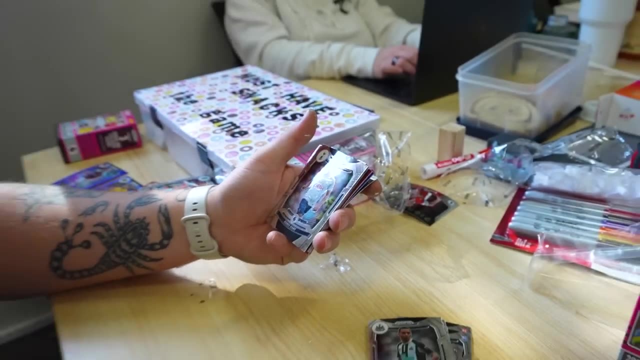 I just needed these. Ooh, I got Jordan Henderson. I'm actually getting a couple good Liverpool players. Those are the ones I'm looking out for. I honestly don't know Whoa. Harry Kane: He's your favorite, Harry Kane. 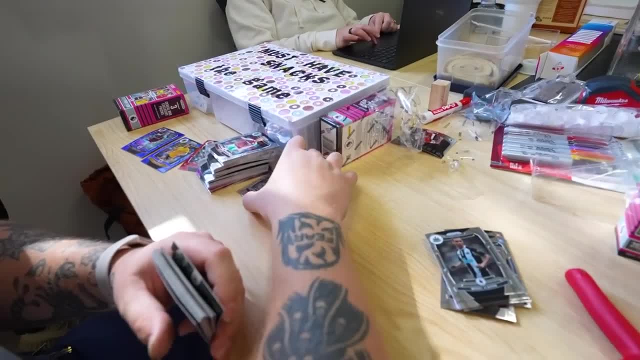 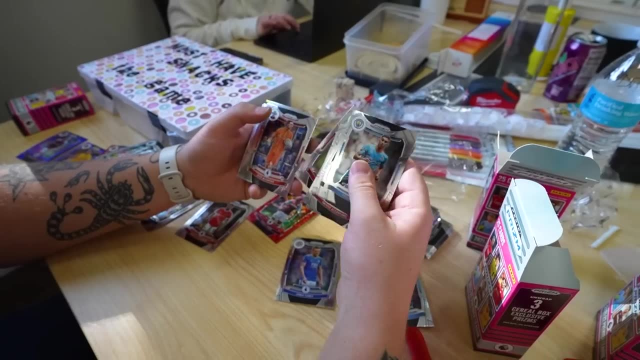 He's not my favorite, but Tottenham is my dad's favorite team, so I'm going to have to give him a high ranking for the game stats. Ooh, Marcus Rashford, Ashley Young- These are some pretty decent players. The most important thing is that I have enough guys in each position, because each team is 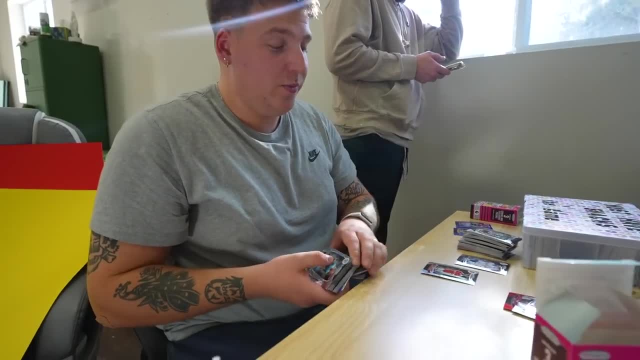 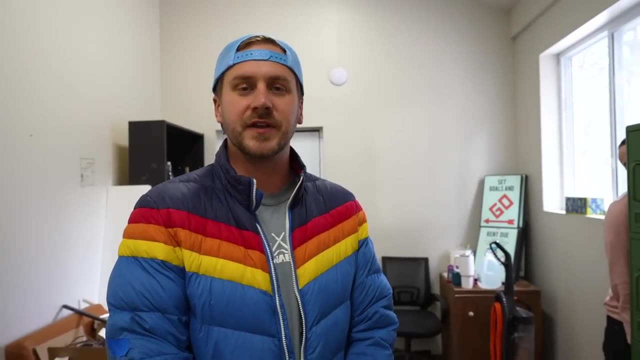 going to need one. I got some cool cards. I don't know every person in the Premier League, so there's a lot of these I don't actually know. I'm making up stats, I'm your guy. Perfect. We are all done with our board games and it's time to introduce you to our judge, Alex. 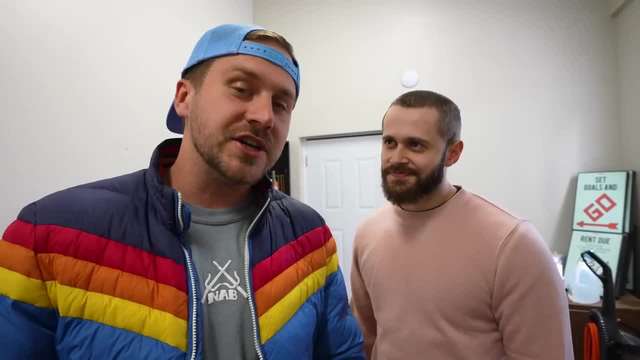 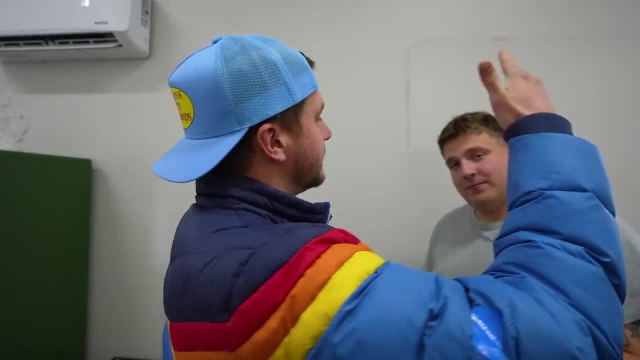 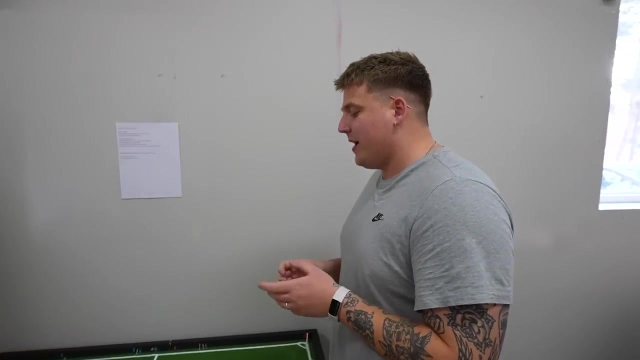 the editor who is going to be judging and determining which of our games is the ultimate board game? I love this kind of thing. First up is Isaac Takeaways. My game is called The Pitch. It is a clean, aesthetic, simple, turn-based sports card game with a sweet game board. 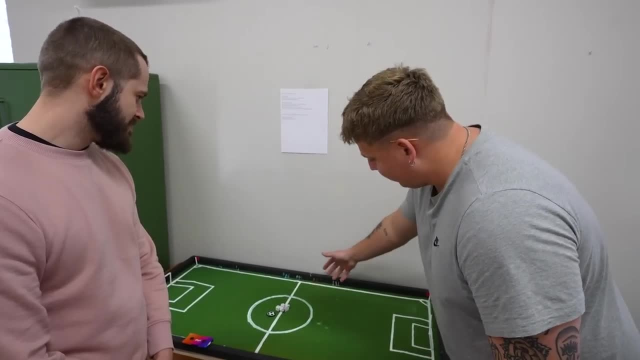 It's a very immersive set. We've got the whole pitch here, We've got all the little guys standing around waiting to watch. So, before we put our teams down, what are your first impressions? I think I like the board a lot. 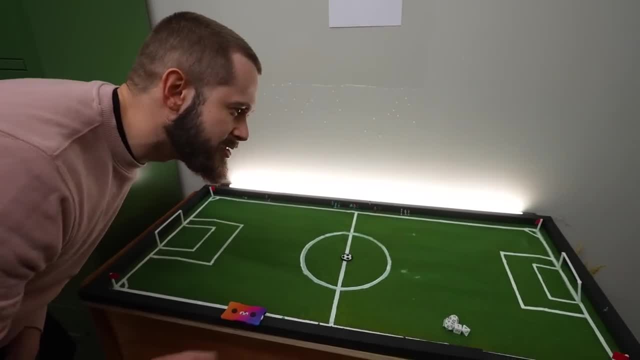 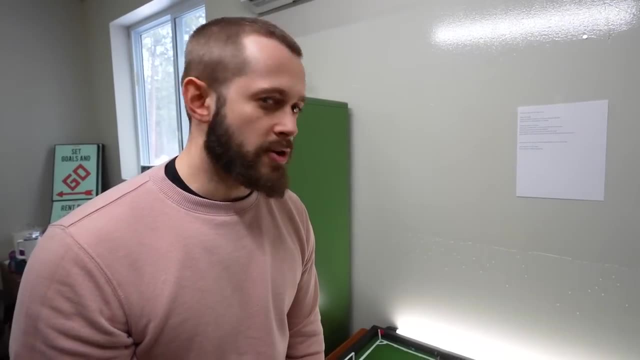 It looks like you spent some time. I like the spectators here. The little details go a long way with me. I like that you made soccer into the ultimate board game, because I am bored when I watch it. But he's already explained the rules to me. 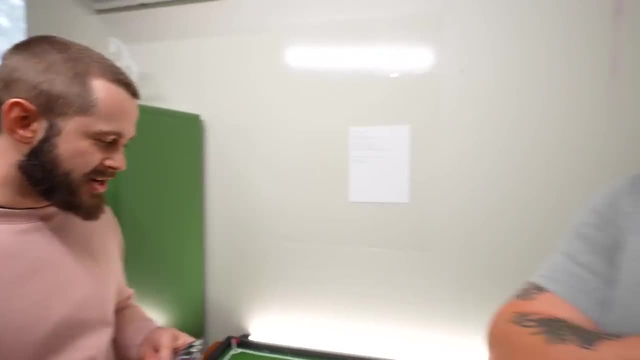 He's probably going to have to walk me through it as we go, but I'm excited to see what's going to happen. I'm going to walk myself through it as we go. Okay, I'm choosing my players at random, All right. 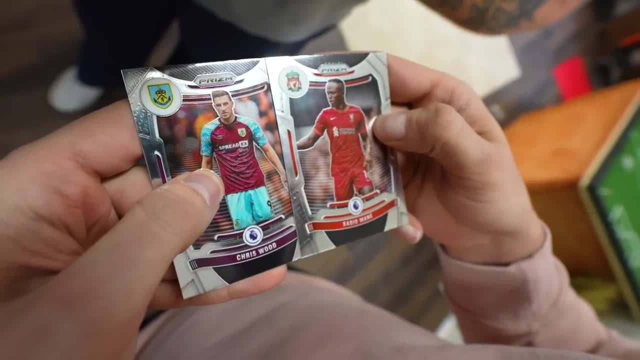 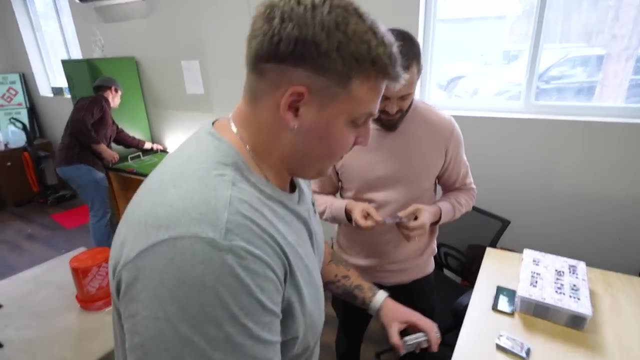 We need two forwards. Ooh, got a guy on Liverpool, That's good- Chris Wood and Sadio Mane. Okay, Those are your two forwards. They're my favorites. Okay, Do I put my cards on the? Yeah, So you put them facing me. 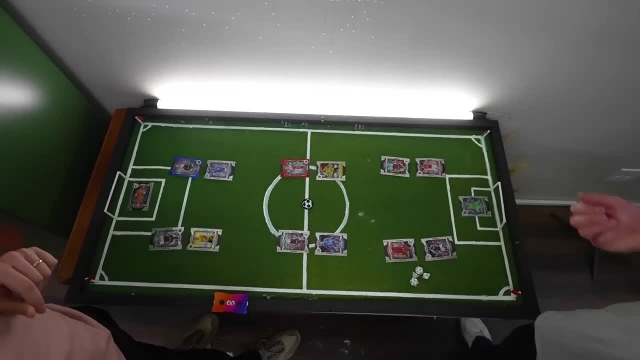 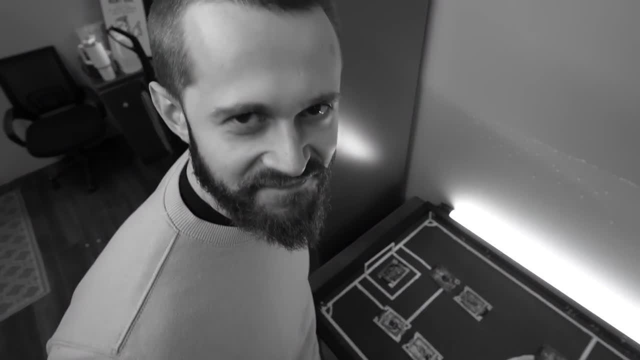 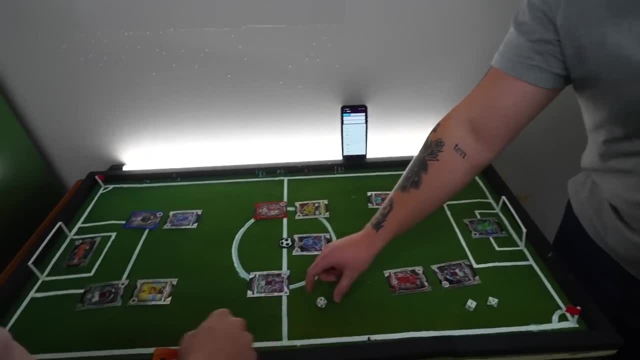 Yeah, So you roll this one. and then you want it to do a hard one. Yeah, So you roll the eight-sided dice. How do I know if I get a red card or not? Well, if yours is lower than mine, then that's a failed slide tackle. 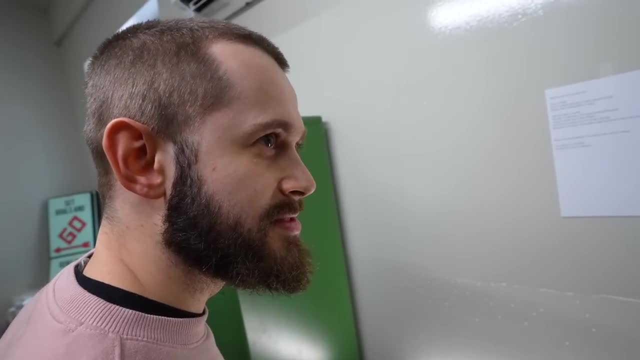 Automatic red card. It's a failed slide tackle. Well, you're getting automatic red card because you're going for the hardest tackle. Oh, so, no matter what, I get a red card for hard tackling. Not if you win, Then it'll be a successful tackle. 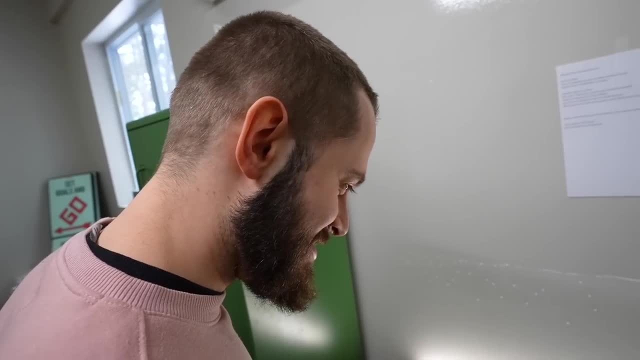 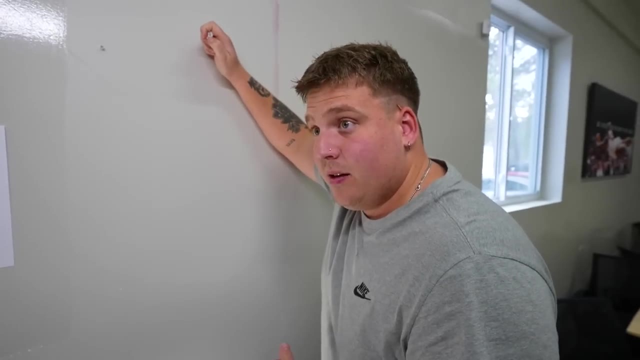 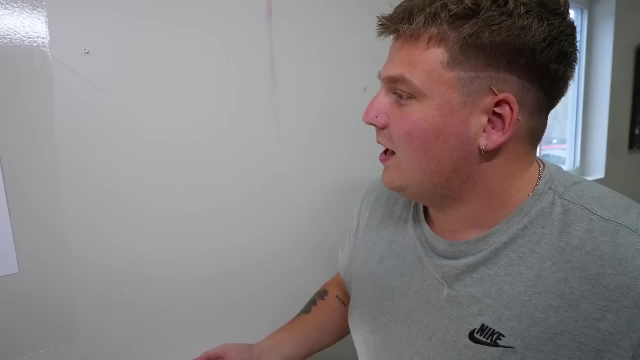 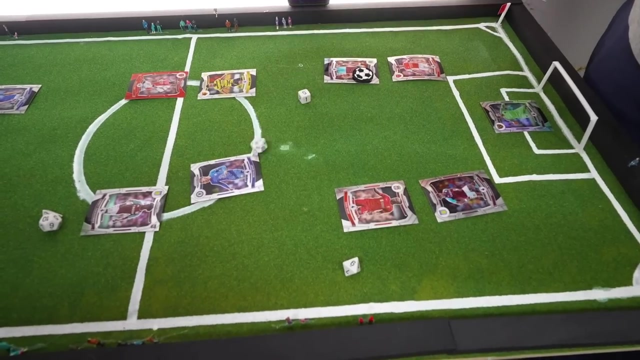 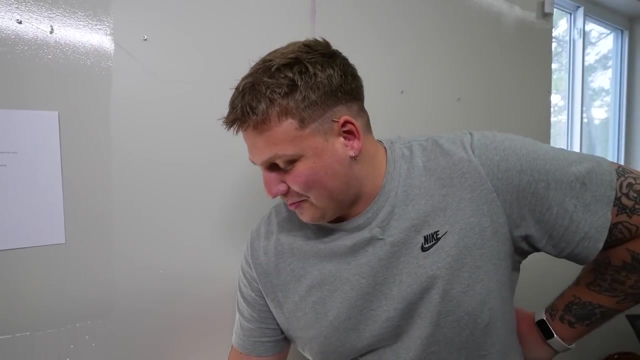 Okay, Okay. So I'm going to, I'm just going to tackle you. Yeah, I'm going to go for a light slide, tackle Nice. Now I'm going to pass up to Mason Mouth again. Dang, am I getting nothing? 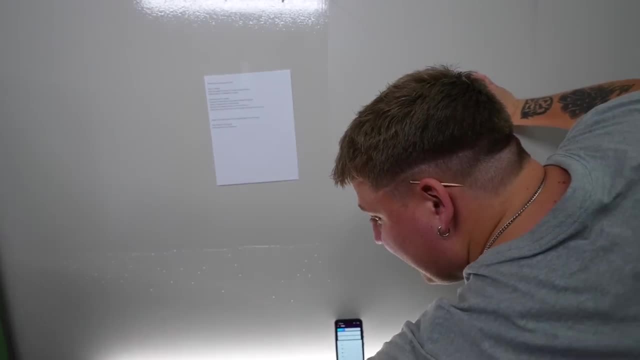 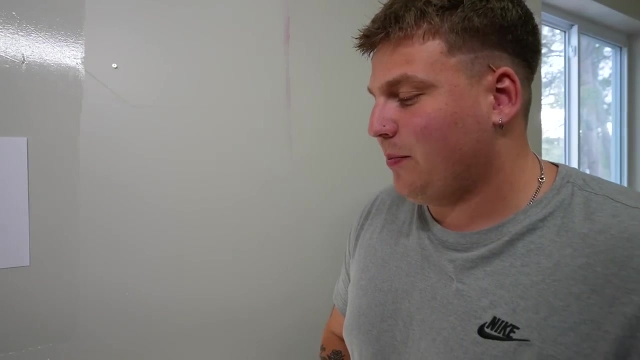 Okay, Nothing. Wow, Does that mean you get a yellow card? Yeah, Oh yeah, yellow card. I don't know what that means. You guys, I'm gonna full send the shot from outside the box. Ooh, Big one 15.. 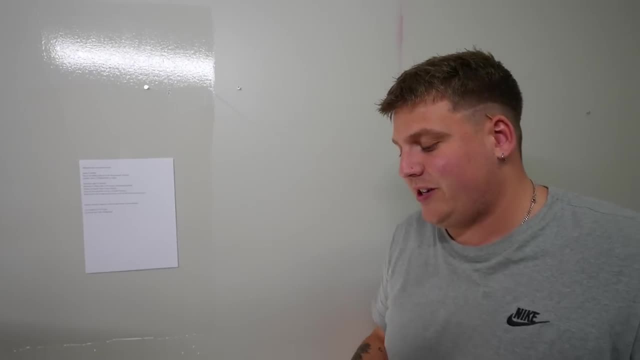 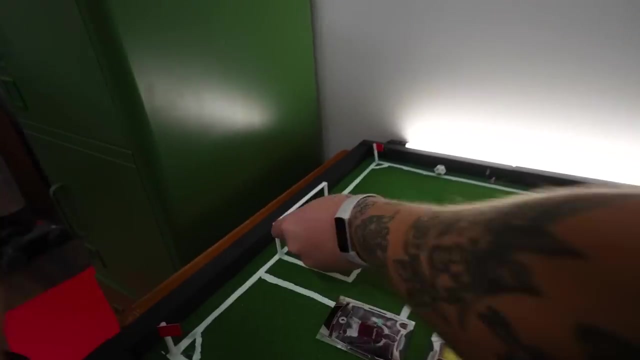 Since I'm shooting from outside the box, you get to roll a six so you have a higher chance of saving since I'm shooting from so far away. Yeah, Goal, Goal, I actually. I see the vision on this one. I see the vision. 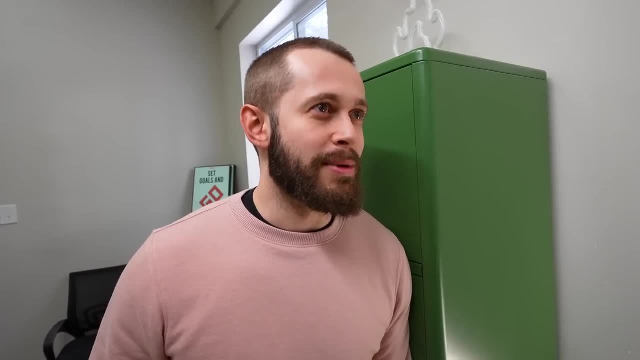 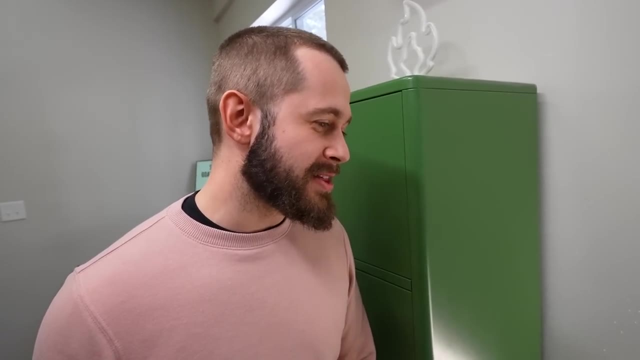 I think if I was an English lad such as yourself- and I was just, I don't know, milling about primary school, I might be able to have a lot of fun with this with my friends. I also think that this is the board you used. 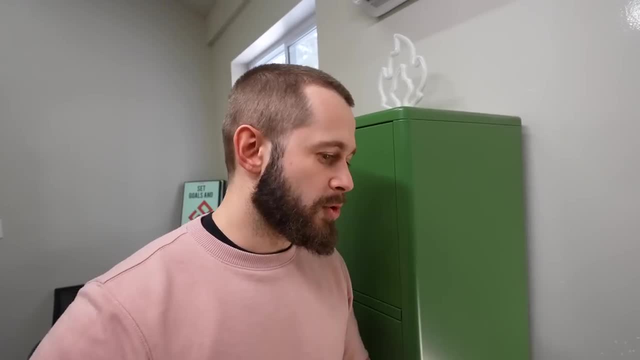 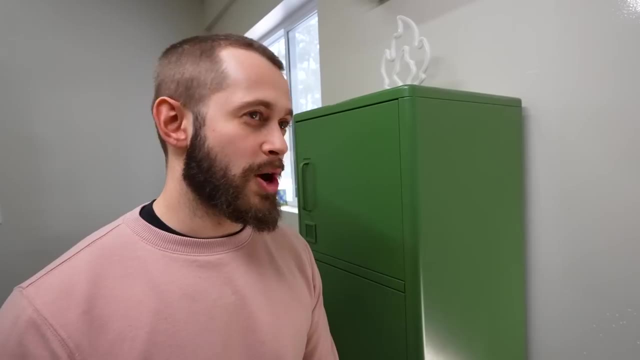 but you could make a version of this board that's a lot more smaller and has more portability, and that might make it easy to play anywhere, And so I actually think a lot of people might have a lot of fun with this. It does have the potential to go on really, really long. 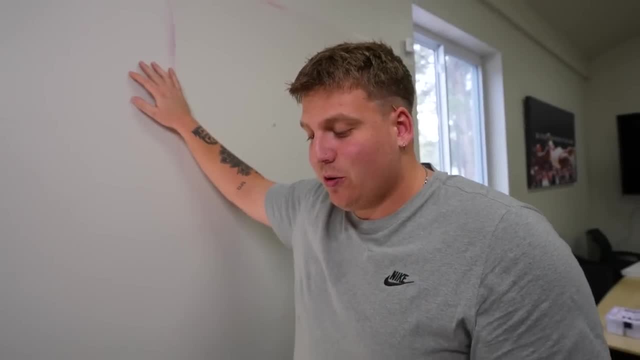 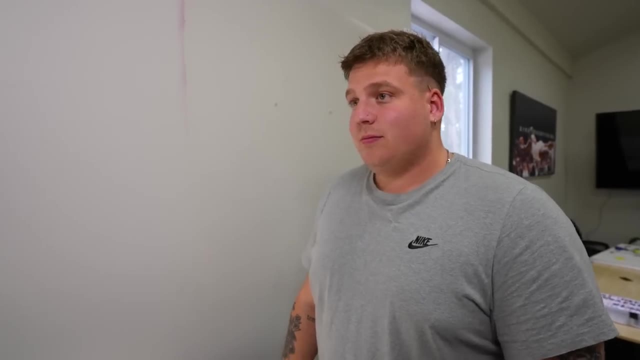 but this game didn't really Like you said. it kind of is supposed to go on long, because football games go along like passing back and forth. It's also slightly like D&D, but with soccer, And so you know if you like sitting down. 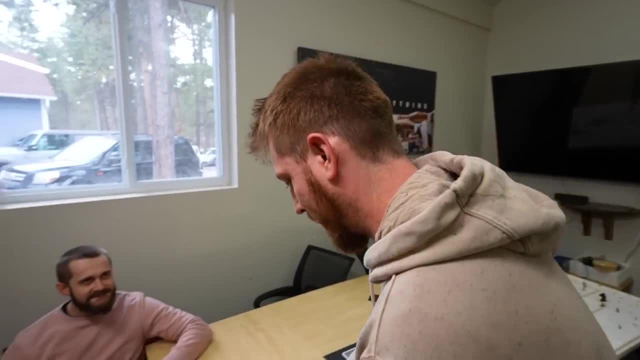 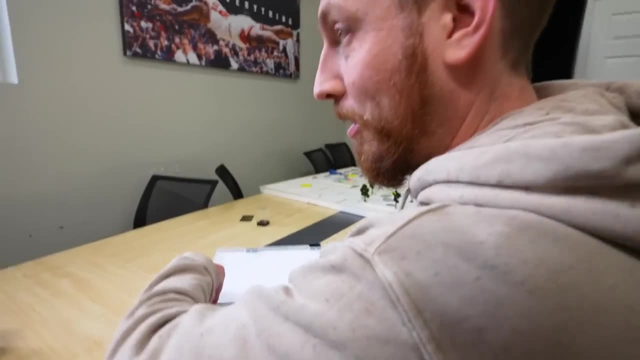 and playing a long board game, then this is for you. All right, Alex, here's my board game. It comes in this handy dandy box, very portable. Oh boy, You like snacks? I do like snacks. Perfect, This is the game for us. 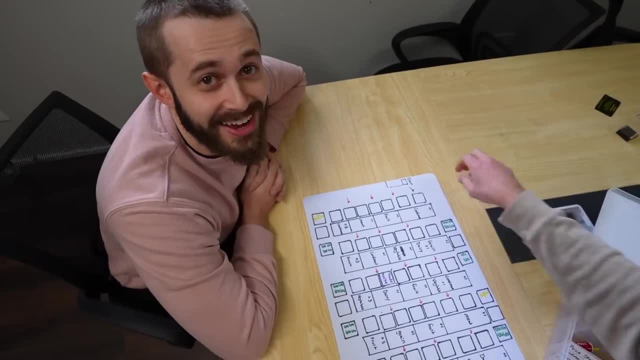 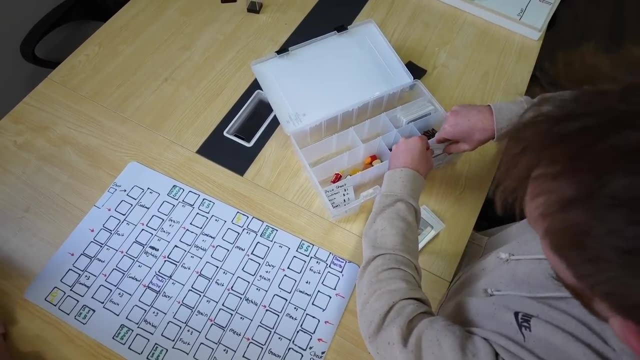 Okay, Pick this game board. Oh my gosh, That is. there's a lot going on there. It's really not that complicated. So the goal is to get as many victory points as you can by completing recipes. So these are what the recipes look like. 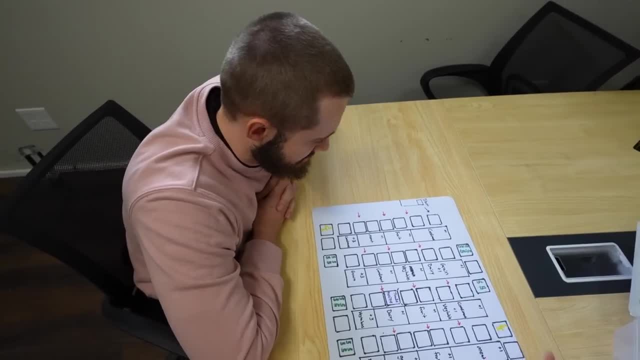 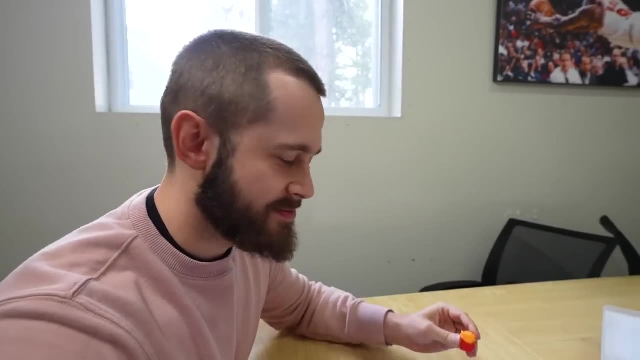 Okay, So you need the ingredients to complete the recipes. Okay, Through the grocery store. Okay, Let's go for it. Do I get to choose a piece? Yep, pick your character. I'm choosing French fries. All right, I'm gonna be hamburger. 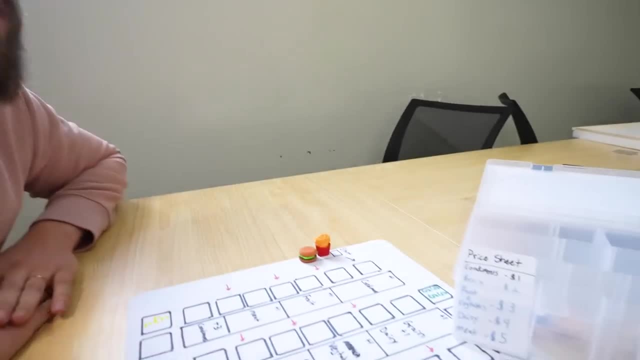 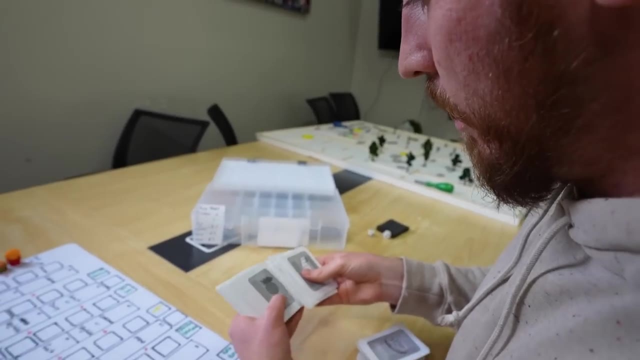 And actually they start on the starting line. It said start and the arrows were right there. so Confusing, that's not good. Oh shoot, All of the ingredients just kind of laid out here. So we've got the milk. 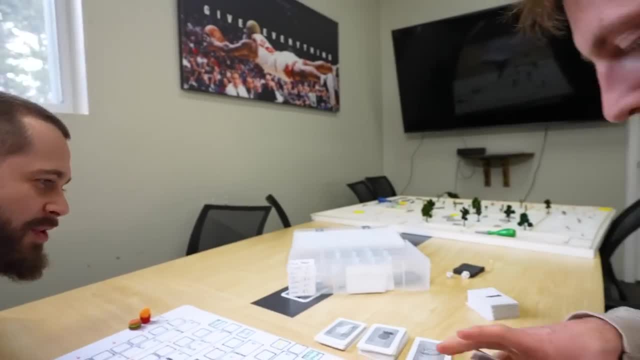 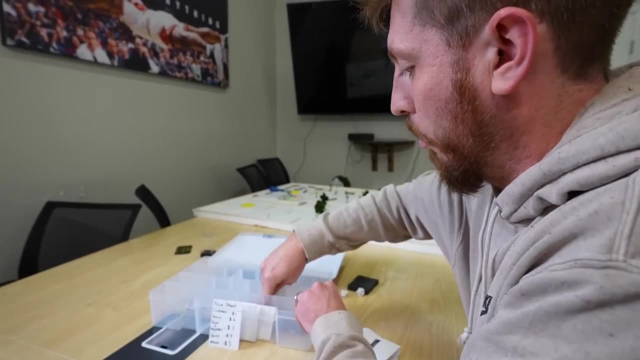 Or the dairy meat, the fruit, the grains. How long did it take you to print off all these different cards? That took a while. Dice. We have the coins here. Coins are important Basically. how it works is you're gonna make your way. 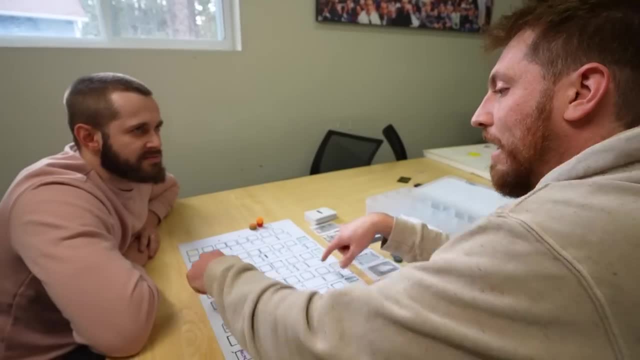 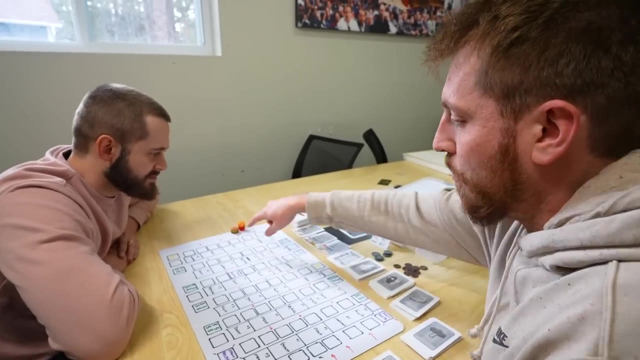 down through the grocery store rolling dice and moving along the board. You can sell back your ingredients if you land on one of the green spaces. That's how you get the money. You gotta use the money to buy your recipes And if you roll a seven while you're in the grocery store, 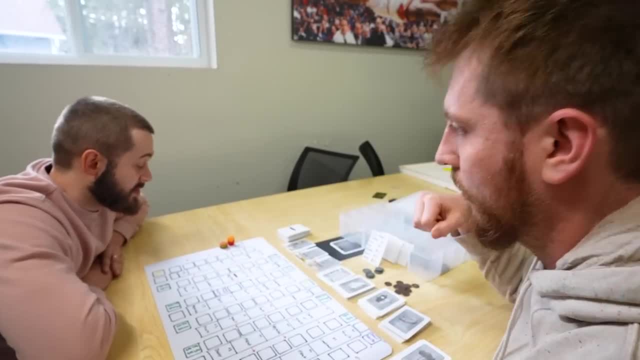 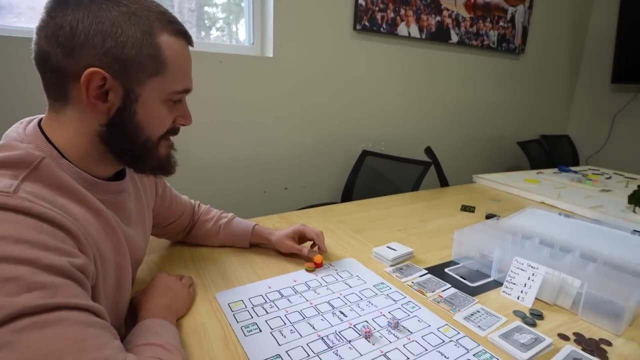 all your ingredients have expired, You put them back and you go back to the start. Oh, give it a roll, I'm gonna roll it. Yeah, Okay, 11. Okay, So you know one, two. it's like that. 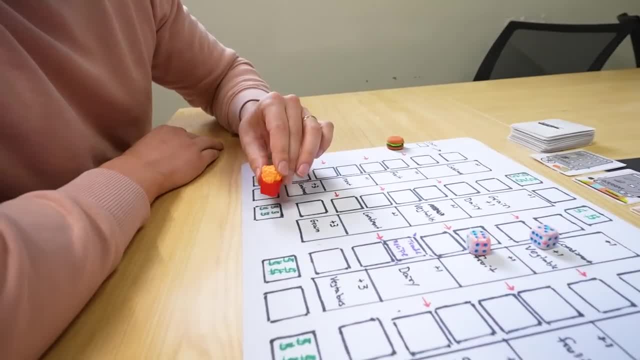 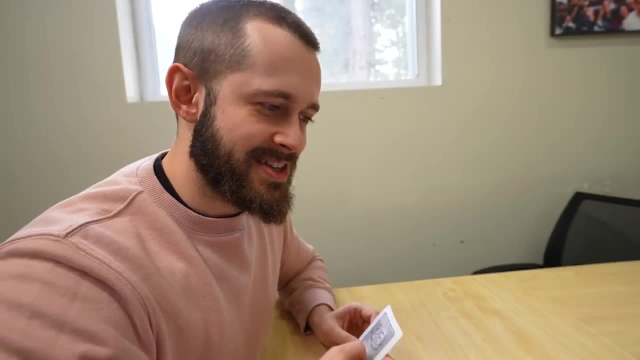 Three, four, five, six, seven, eight, nine, 10,, 11? Plus three grain. Wow, big time. There you are, Nice, All right, what do I think? Ah, All right, condiment for me. 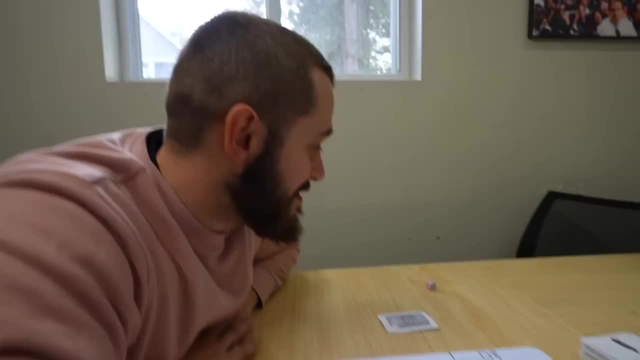 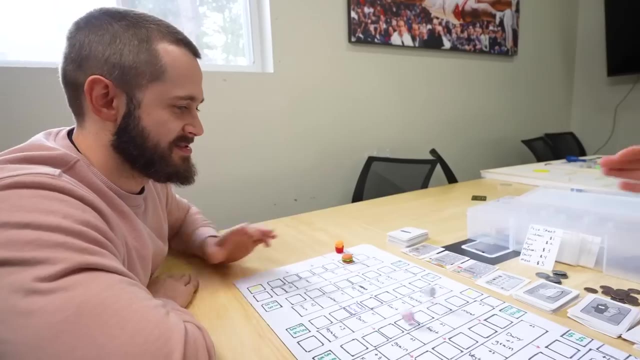 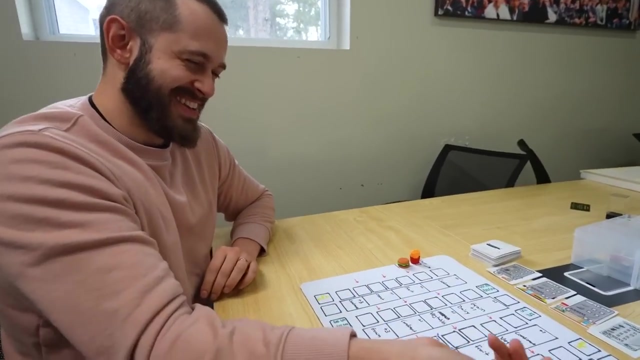 All right, your turn. All of seven yikes. That sucks. Your bread expired extremely fast. You're back to the start. What kind of grocery store is this? It's Africa. Well, my custard expired quick, Okay 10.. 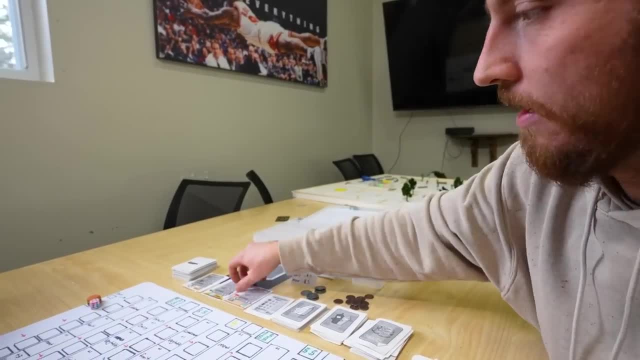 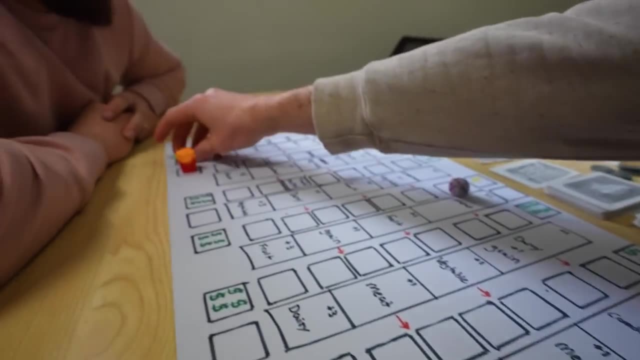 Now see, if you had something to sell, you could sell it, But since you don't have any ingredients yet, it didn't really work out for you. Whoops, whoops. So I should be right here. Wait, Oh, that's a concrete condiment. 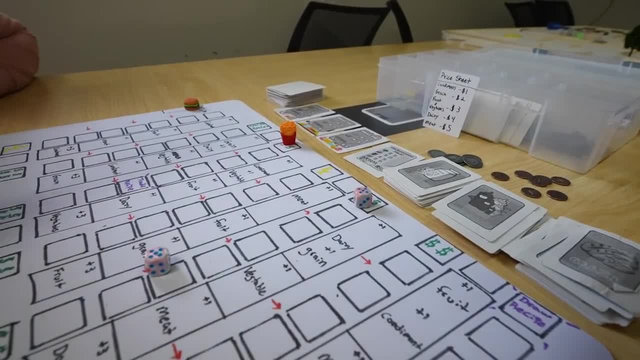 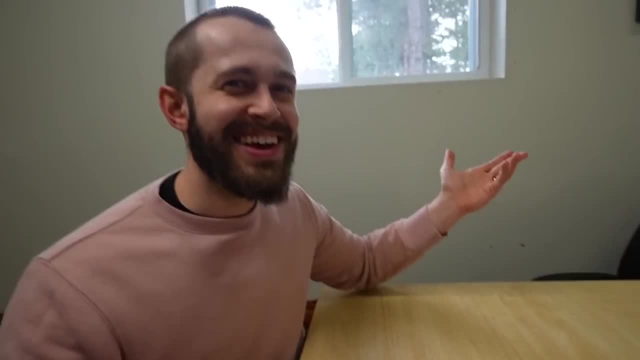 10. Again, I keep landing on the money One, two, three, four, five, six, seven, eight, nine, 10.. This whole time I've only been on money stuff, so I haven't gotten any ingredients. 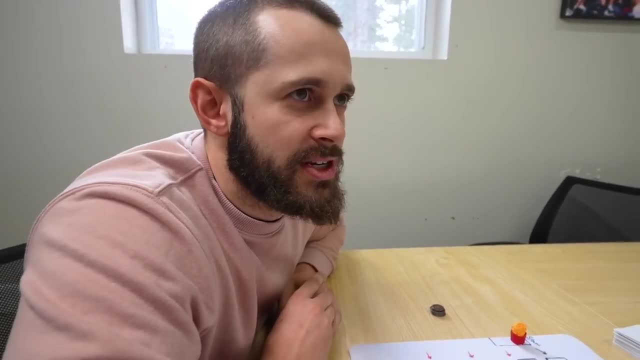 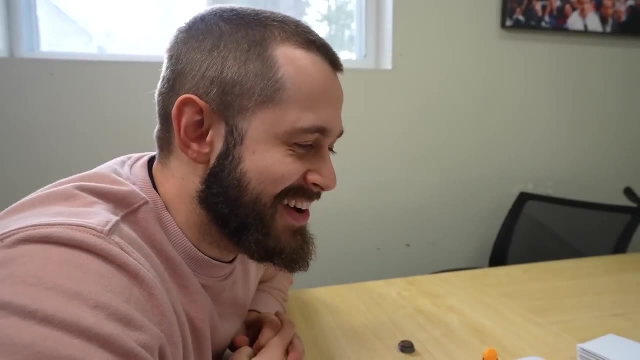 One eternity later, At what point do I have enough money to buy a personal chef to just make this for me? I don't see it on the price sheet, but that could be an expansion. Yeah, we should expand it right now. You know, if we had some grocery store stuff? 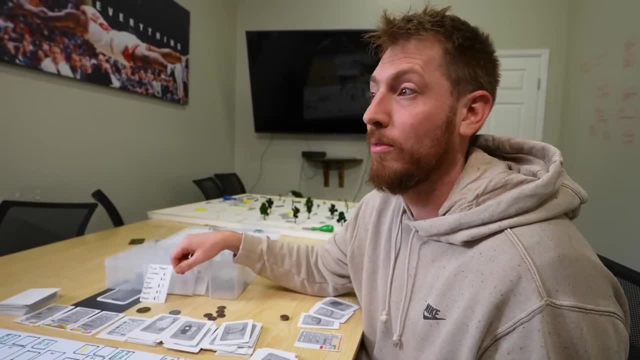 we could just make this for myself. If we had some grocery store music playing, that would really enhance the vibes too. you know, That's true. Oh, oh yeah. No, sorry, I'll do it, I'll add it in. I'll add it in right now. So all these recipes have victory points. so once you get 18 victory points, you win the game. How long do you foresee that taking? Uh, it depends on the players. Around 30 minutes for two-player. 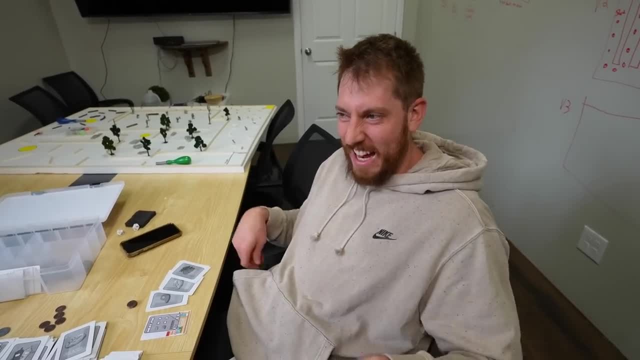 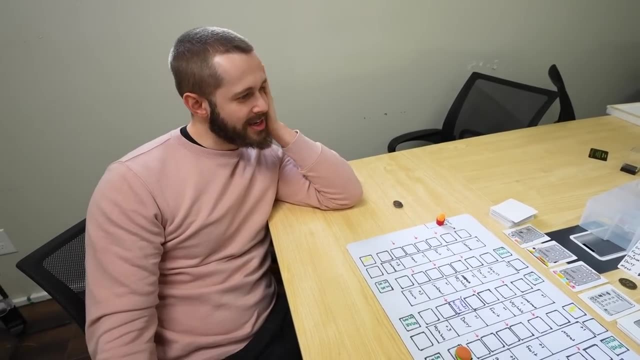 maybe around 45 minutes for a three-player game and it just kind of adds from there. Okay, The board is not very- It's not very fun-looking. It kind of looks like a breakdown of a tax sheet or something. I don't know why this would come to mind. 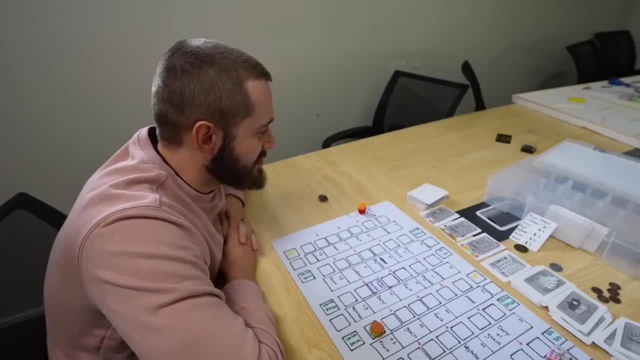 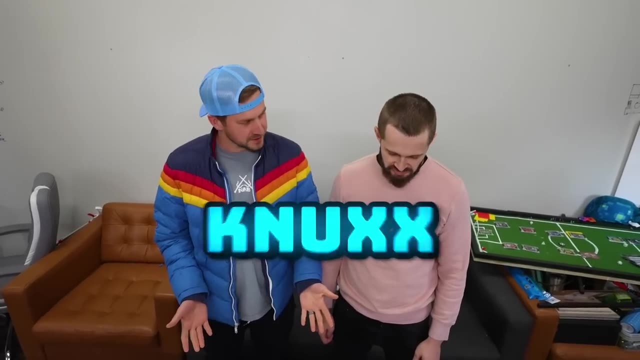 Could use some more color, Could use some graphics, maybe. Keep in mind this is just a prototype. Right, Make sure the game worked. Yeah, the game works All right, Alex. this is Nux, an interactive race game. 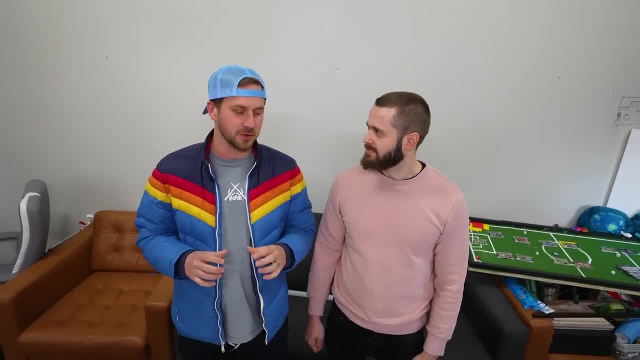 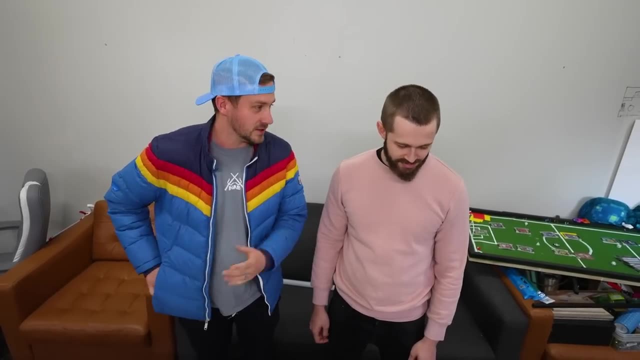 It's fun for the whole family. My favorite type of games are the simple games that don't require much thinking, but you also get to use your hands and there's a lot of like variety. So it's as simple as any race game. 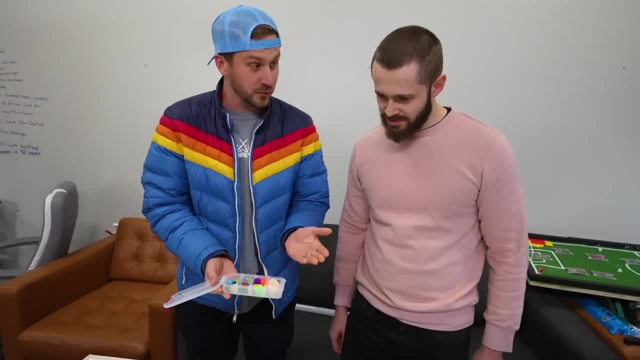 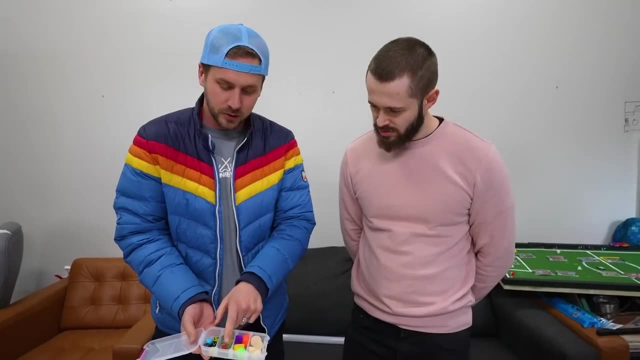 My game comes with four different types of racers. These are your racers, So we are going and taking turns to see who can get to the finish line. So we got marble, these glass, different shapes, little soft guys or these things. 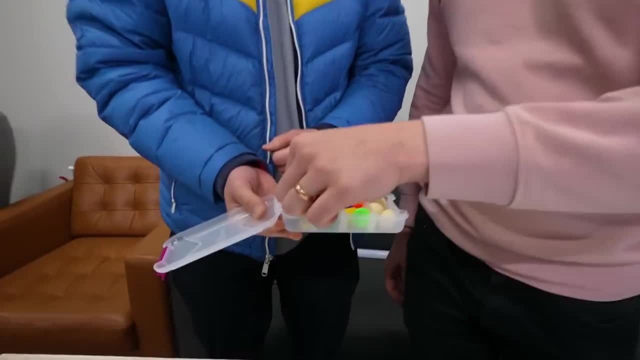 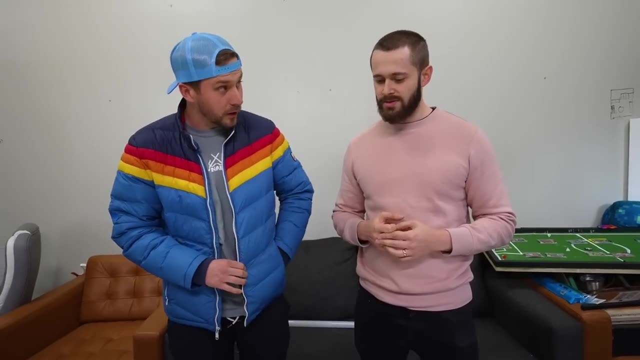 My favorite is the marble, so we'll. I was gonna say that seems much faster than all the other options. We'll do that first. It's called Nux because you use your knuckles to hit the marble around the course. or you got the expansion pack. you use these little. 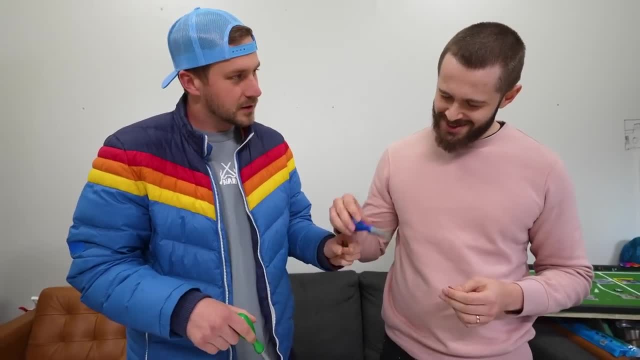 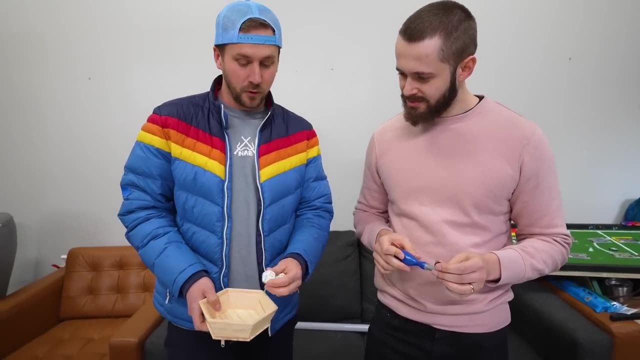 hitters and you can use them to. What are these? They're just paint brushes that I cut the tip off. Oh, okay. Another variety of the game is I have these dice that go up to four, so we each will roll every time. 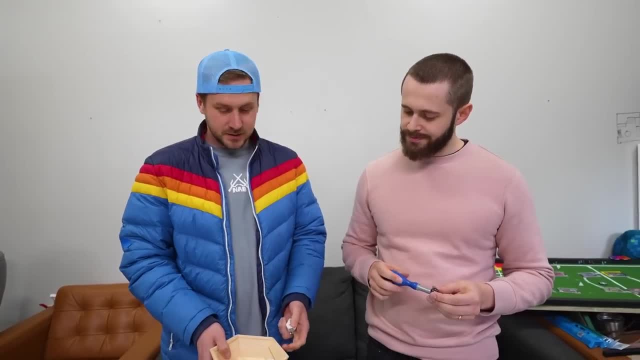 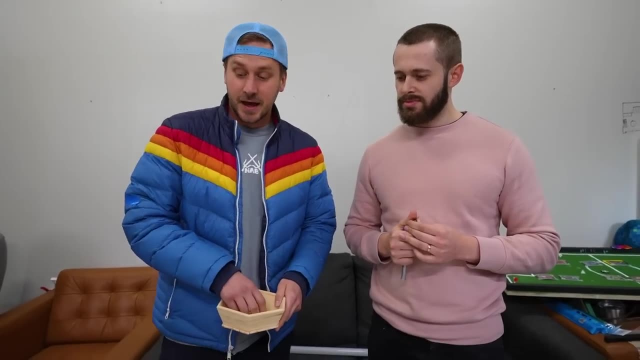 That means you get to flick it four times. Oh, okay, You choose to use this or not. You can just take turns doing one hit at a time, but I thought this will add good variety and change And one little bonus if your marble lands in these. 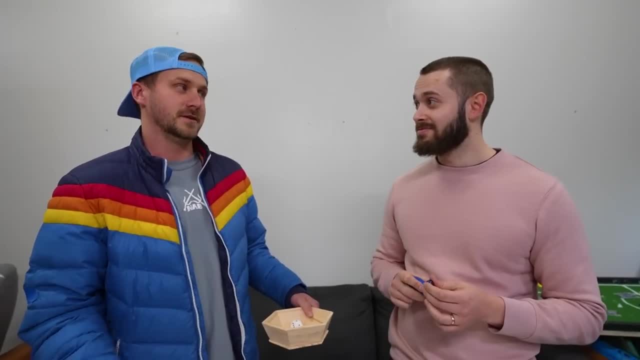 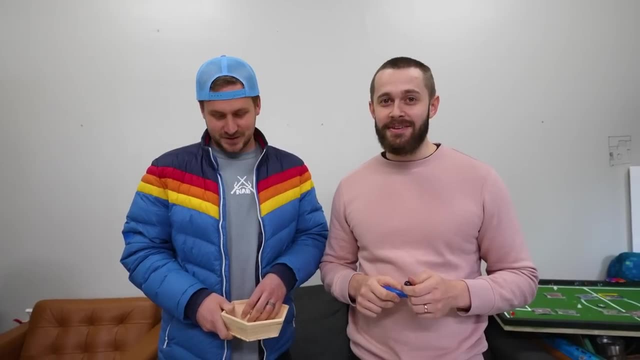 that is the Nux zone, And if you're a fan of the channel, since you edit all the videos, you know exactly what that means. Oh no To Nux your opponent. Oh no, That is scary. I have Nuxed someone, but I have never been Nuxed. 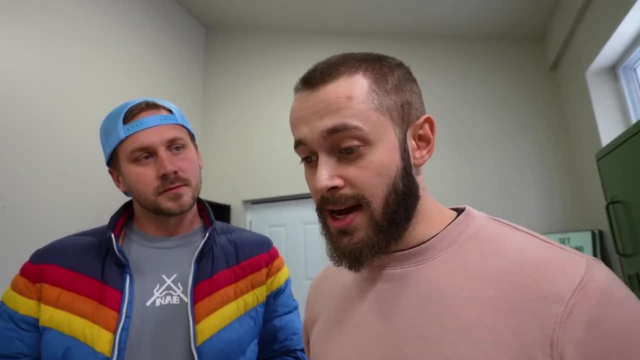 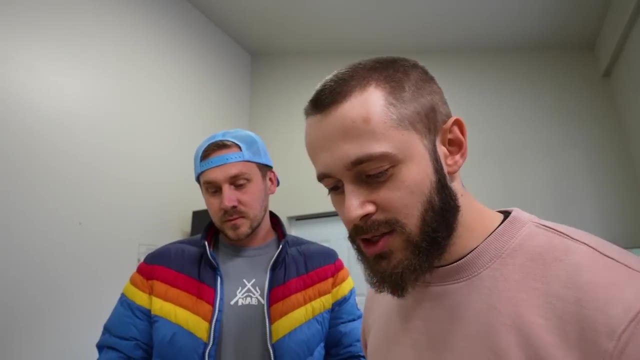 Any initial thoughts before we play. I like it. I like it. A lot of time went into creation, the gluing of the pieces, a lot of details, which goes a long way with me. Are these walls? is it against the rules? 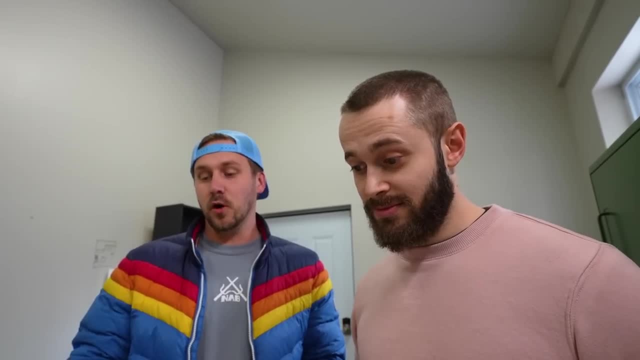 to accidentally go over them. Yes, so if you flick it too hard, you don't wanna go over the walls? Do you get Nuxed if you go over the wall? That is a great rule that I didn't know. I didn't think about it. 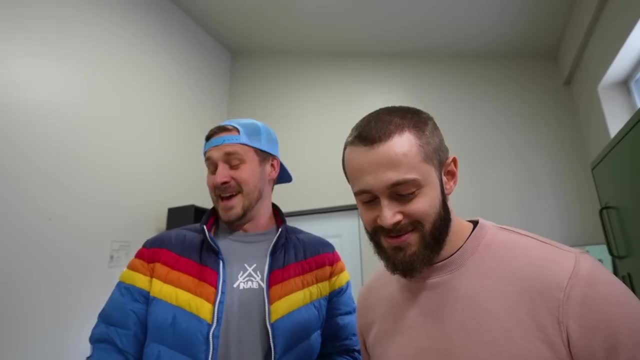 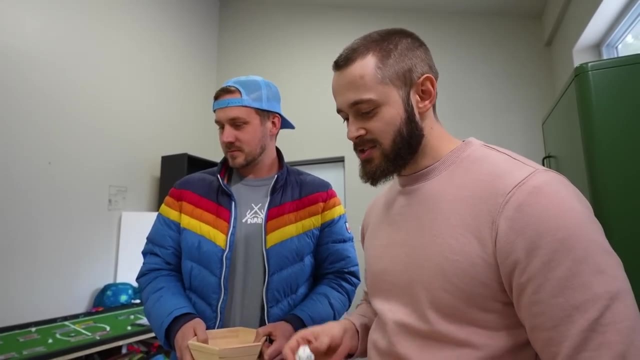 I like that rule. Yeah, so I might be unconscious by the end of this game, but Yeah, Well, you'll see it just throughout. we have different kind of levels, a lot more obstacles at certain points, Okay, okay. 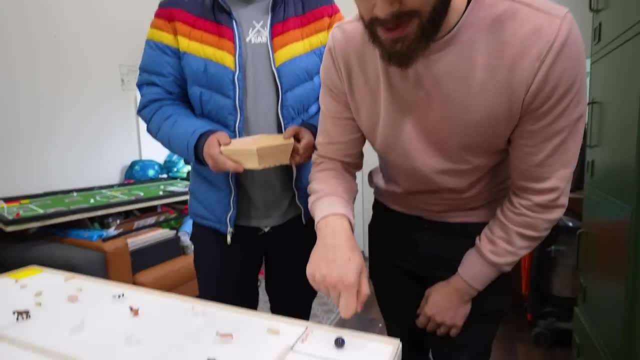 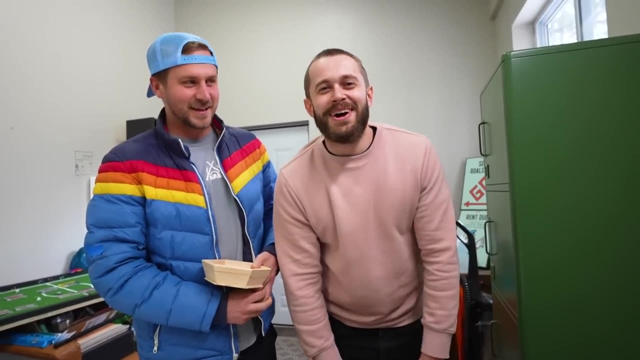 So I'm gonna roll see how many Nux I get One. all right, that's not what I wanted, but All right, that's. the journey of a thousand miles begins with one step. you guys Three Well. 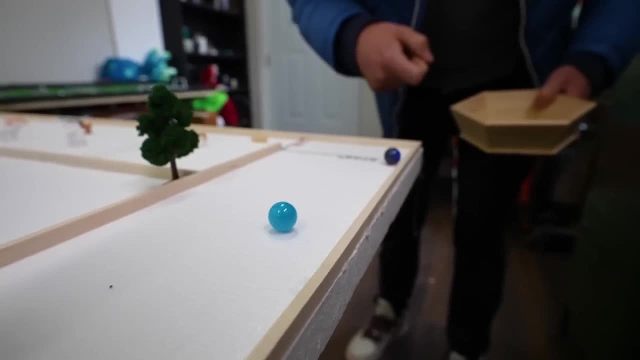 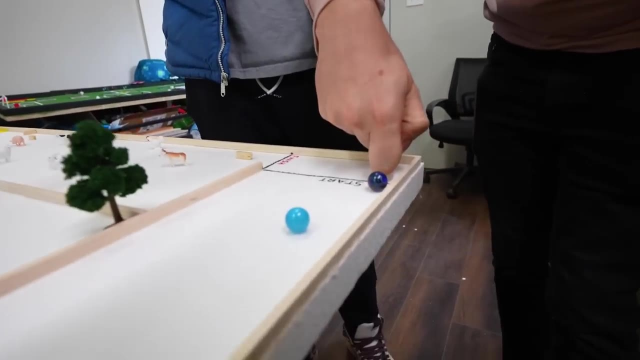 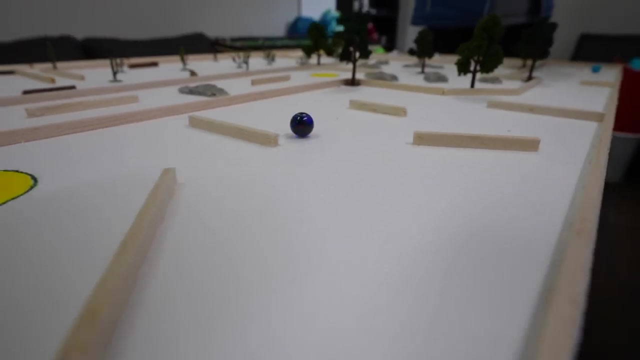 That was worse than mine, Surprising. Yeah Two. Oh, It takes actually skill to play this game Right, So not just full chance. Two more. I wanna Nux him. Oh, that was close to the Nux zone. 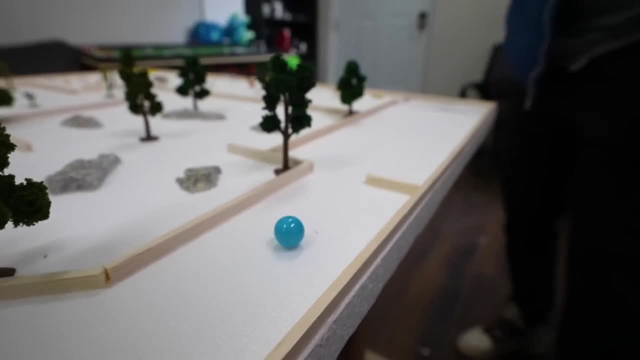 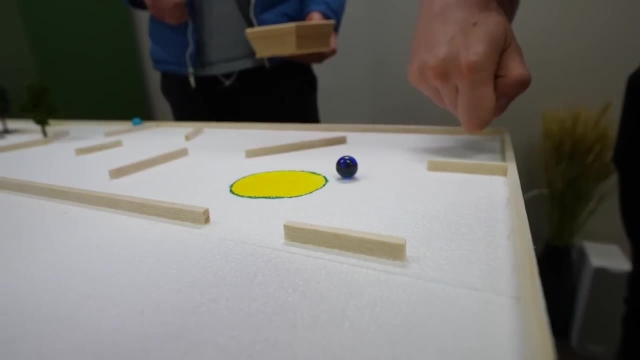 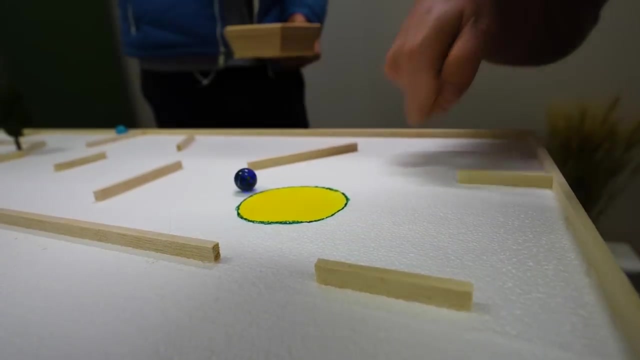 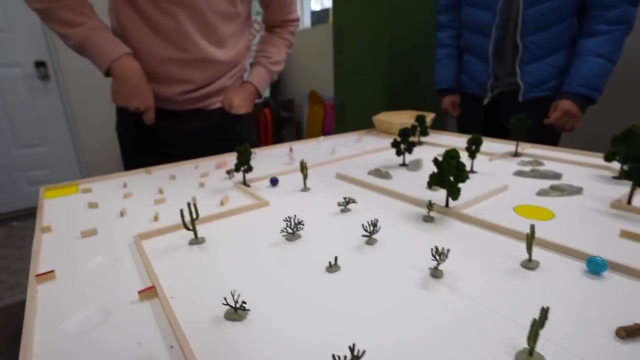 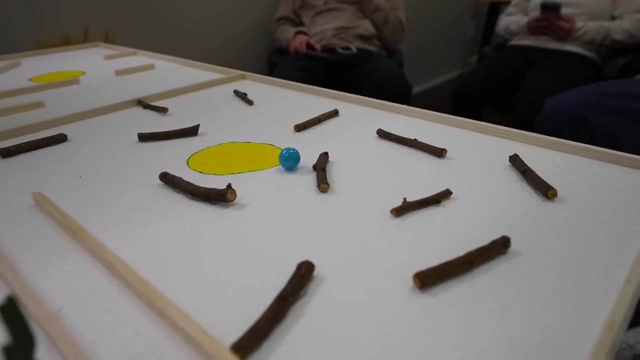 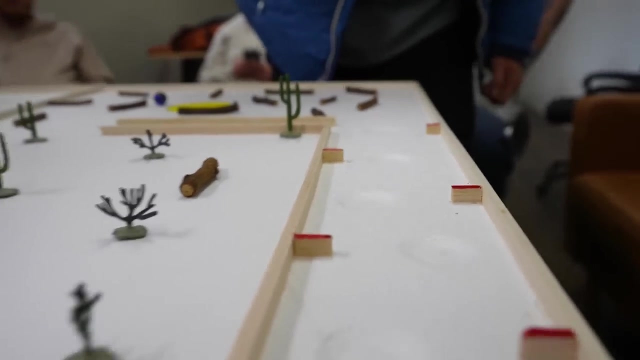 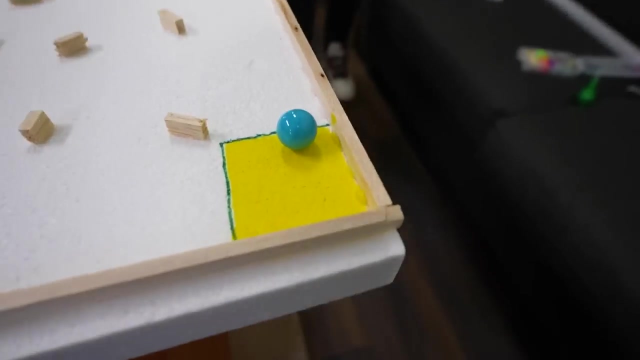 Oh gosh, It has to stop hanging. Oh, you're really wasting your roll to do this. Yes, No, Yes, Yes, Awesome, Brutal. It could change at any time. Oh Dang it. No, No. 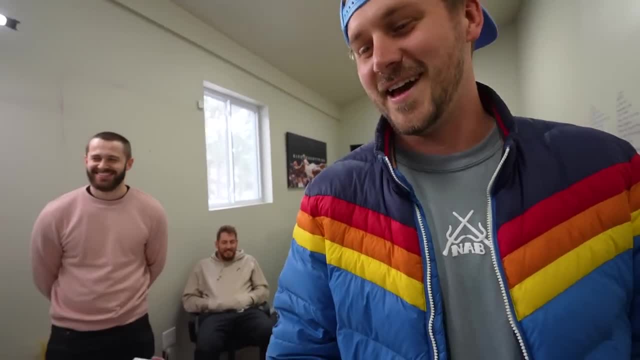 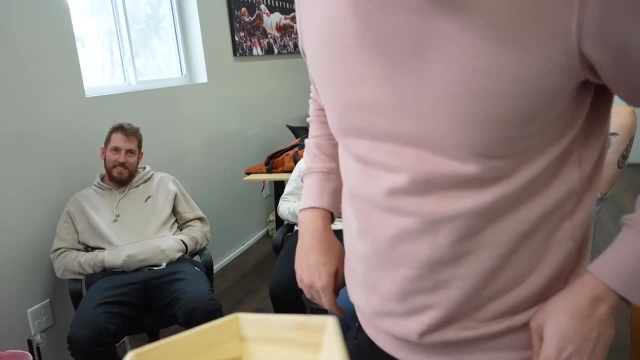 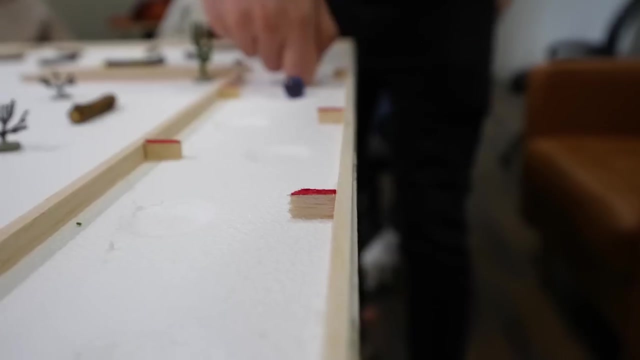 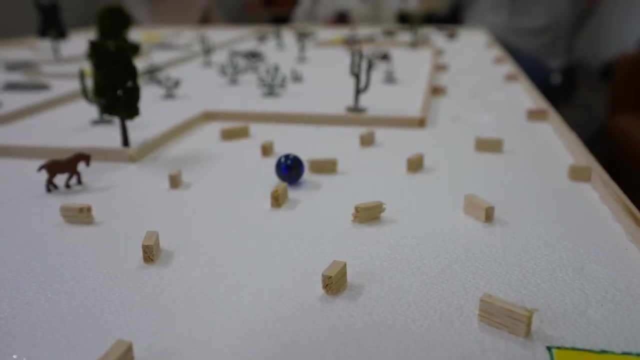 Yes, Dang it. Ah, Final, Oh, I need a four, Four. finally, Oh, it's in a little crater, That actually might help me. Oh nice, Okay, Three, Two, One, Dang it. 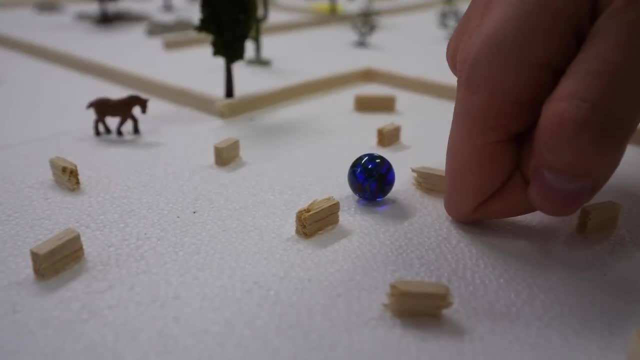 Three. I have to. I have to send it. you guys, The chip shot. Oh Oh, What happened? Nux, It's a Nux. I'm gonna spare you. Are you gonna spare me? We wanna see the Nux. 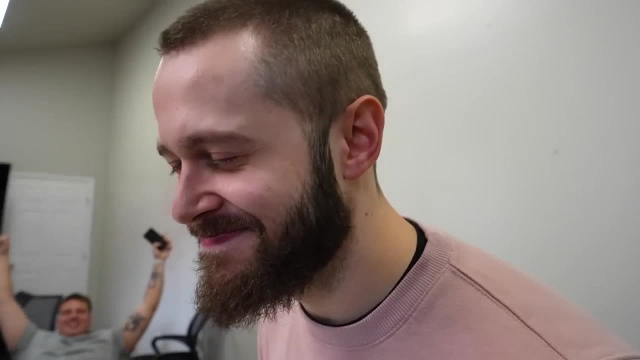 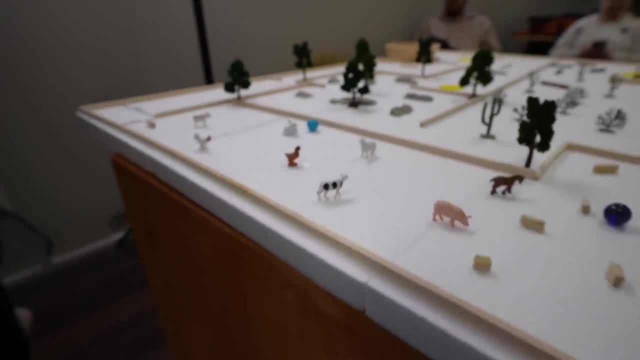 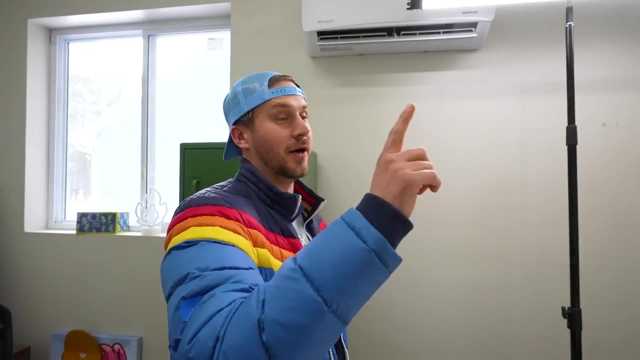 Do the Nux. They're here for the Nux. Yeah, Give the people what they want. Yeah, Yeah, Yeah. Nux Three. Oh, Yeah, Oh. Now that was a two-player game, but if we wanted, we could play four players.